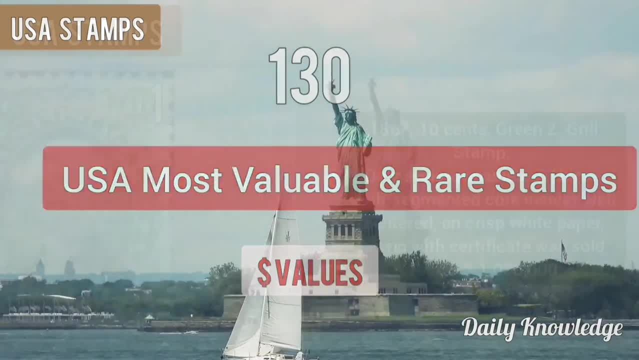 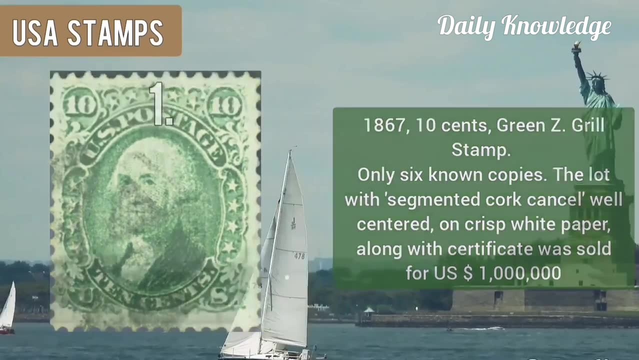 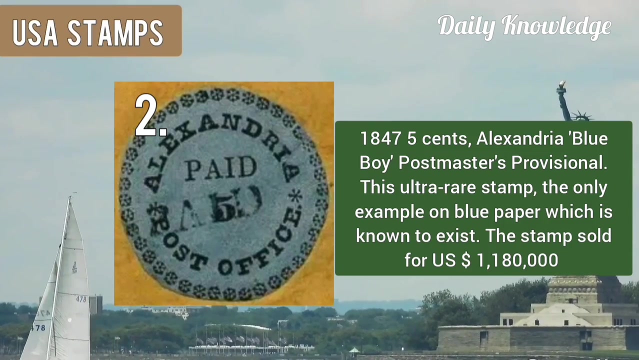 Welcome back. This video is about 130 USA most valuable rare stamps: 1867, 10 cent green Z grill- Only 6 known copies and this is well centered. Next is 1847, 5 cent Alexandria, blue boy post masters, provisional. It is ultra rare. 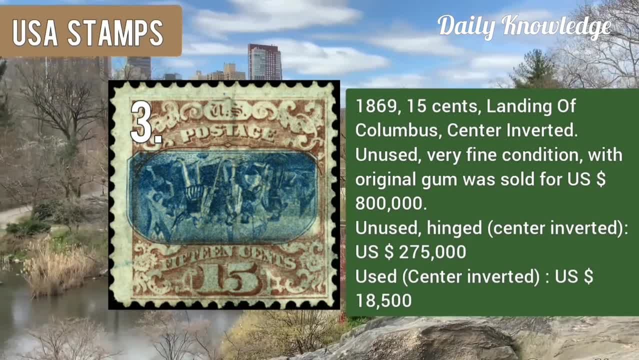 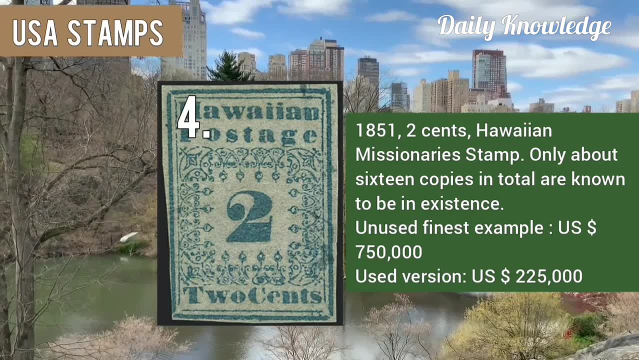 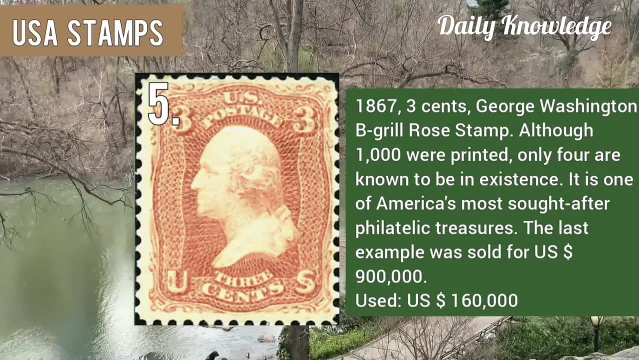 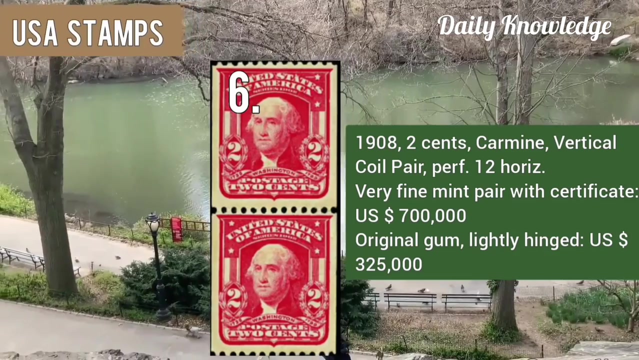 1869, 15 cent landing of the Columbus with center inverted. It is unused and very fine. Next is 1851, 2 cent Hawaiian missionary stamps and only about 16 copies in total are known. Next is 1867, 3 cent George Washington. It is B grill rose stamp and only 4 are known. 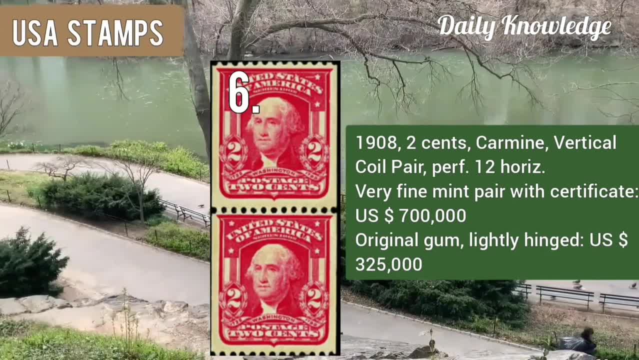 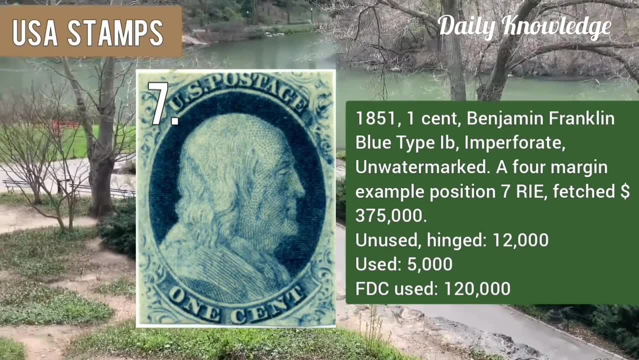 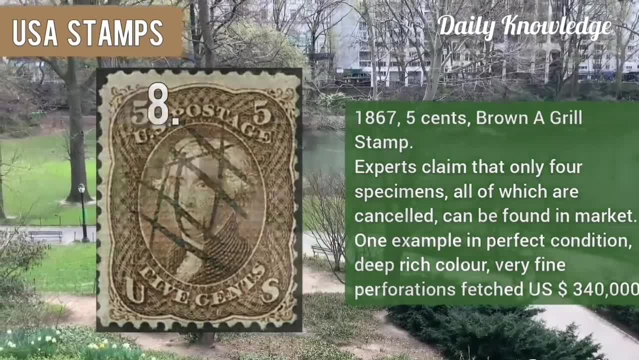 Next is 1851 1 cent Benjamin Franklin, blue type 1B. It is impoverished. Next is 1851 1 cent Benjamin Franklin, blue type 1B. It is impoverished. a grill and only four specimens are known. 1867, 15 cent abraham lincoln, and it is extremely rare. 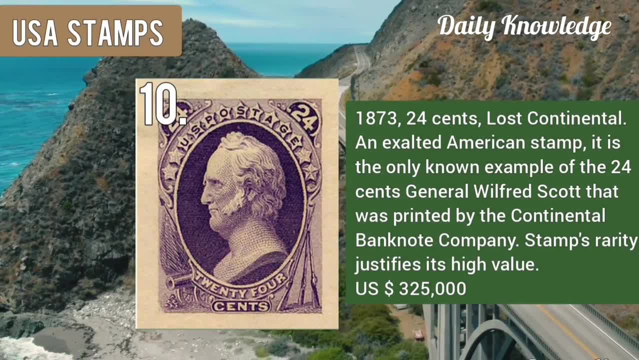 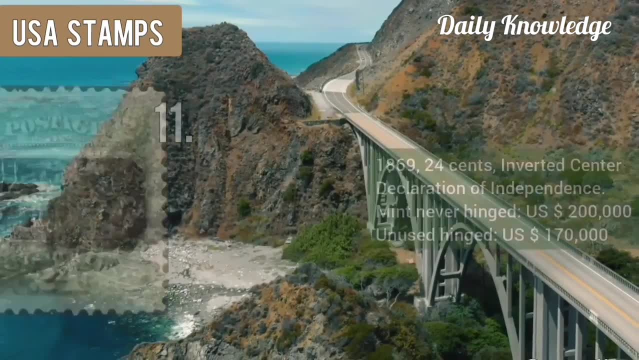 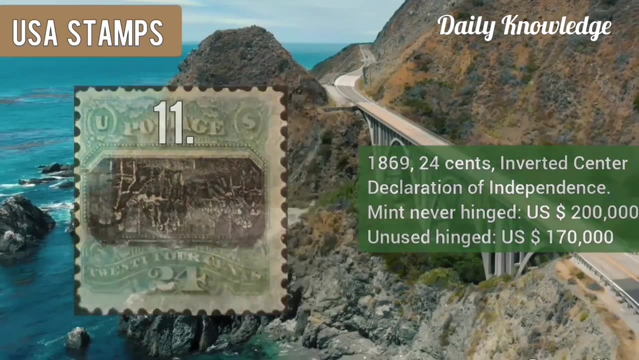 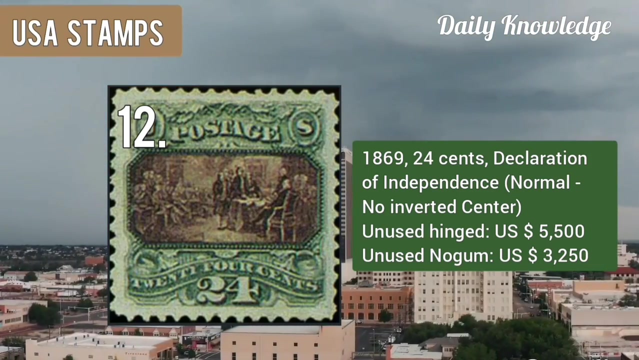 secret that has distinctive horizontal reaches. 1873, 24 cent, lost continental, and it is the only known example now. 1869, 24 cent inverted center, declaration of the independence, and it is mint never hinged. 1869, 24 cent declaration of independence, normal, no inverted center. 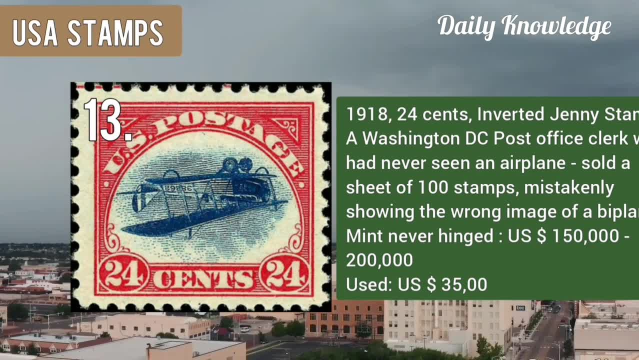 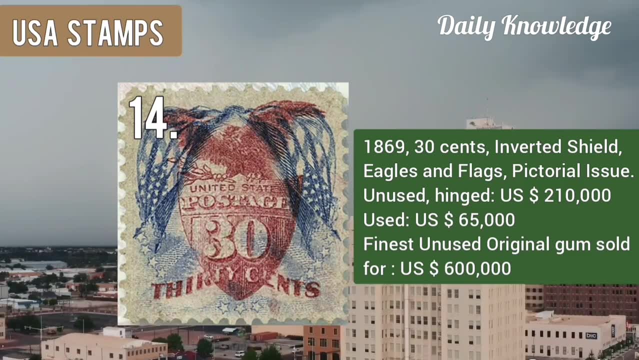 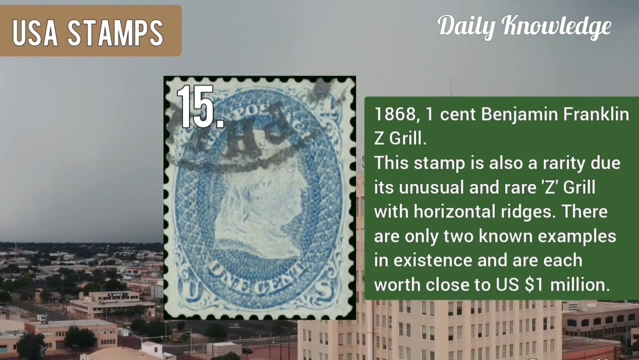 now this is 19, 18, 24 cent inverted jenny, and only hundred stamps were sold in. this is the value of mint, never hinged. 1869, 30 cent inverted shield, eagle and flags. victorial issue, unused and hinged. now this is 1868, one cent benjamin. franklin c grill. 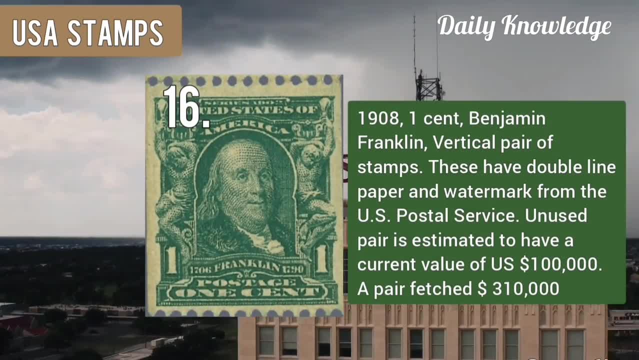 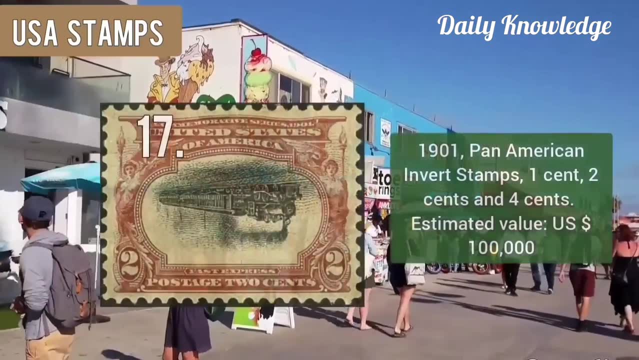 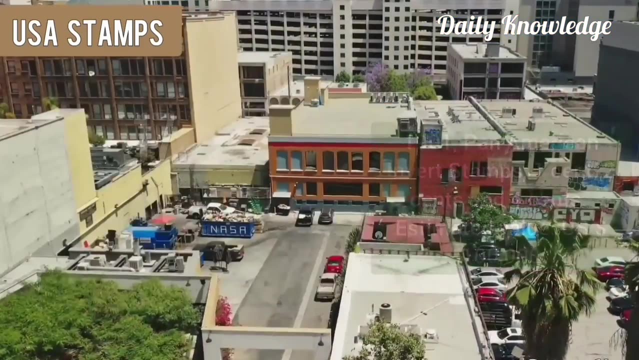 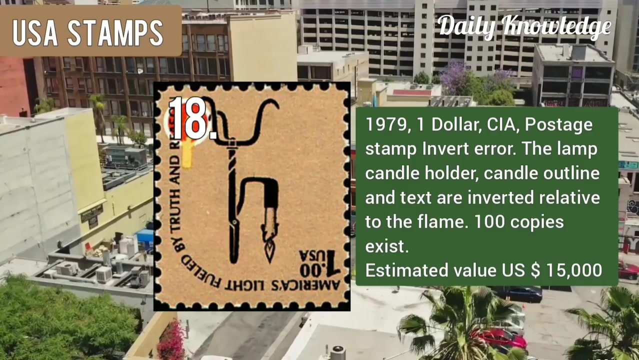 and there are only two known examples in existence: 1908, one cent, benjamin franklin, vertical pair of stamps and these have double line paper. now this is 1901: pan american inward center. one cent, two cent and four cent estimated values. 1979: one dollar cia postage stamp. in word error and only hundred copies exist. 1992, 29 cent. 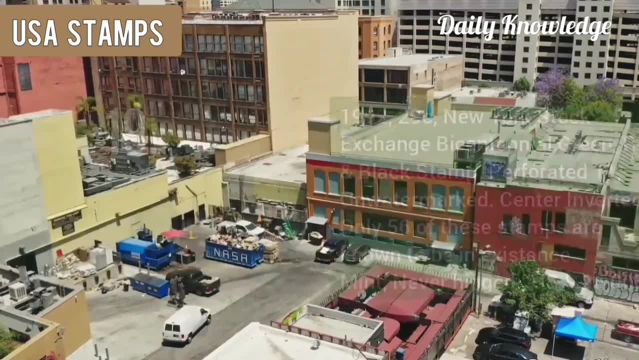 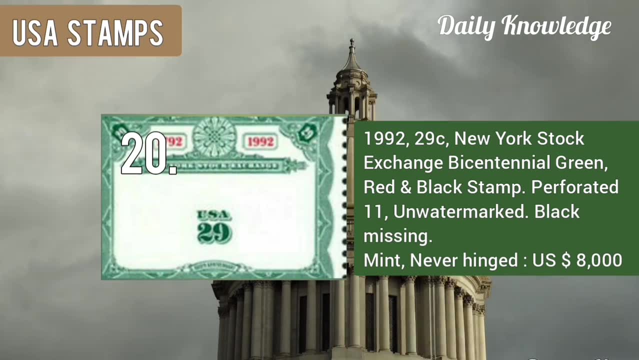 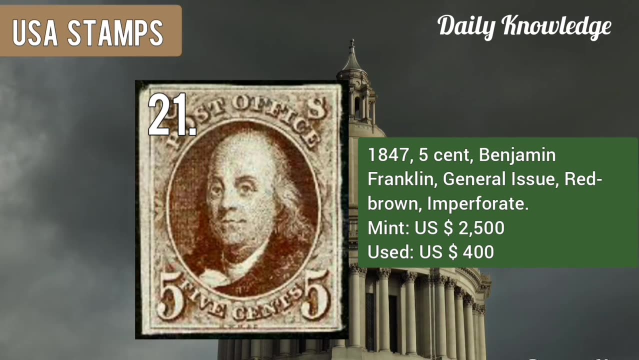 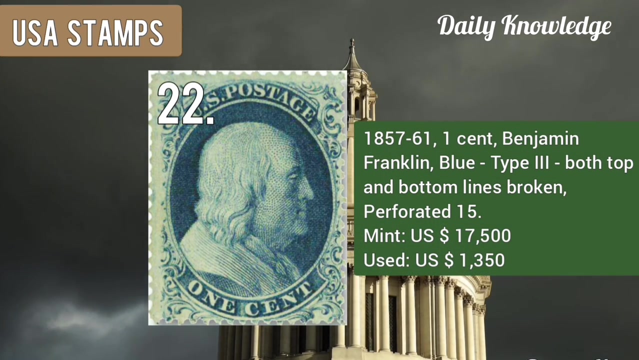 new york stock exchange by centennial green, red and black stamp 1992, 29 cent. new york stock exchange by centennial green, red and black stamp perforated now 1847. five cent benjamin franklin general issue red, brown in perforate now 1857: 261. one cent benjamin franklin blue type three. both top and bottom lines are broken. 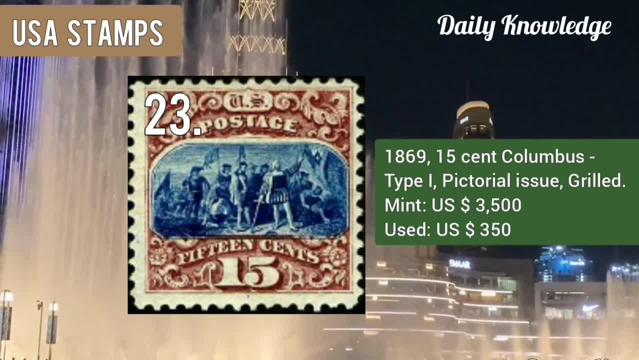 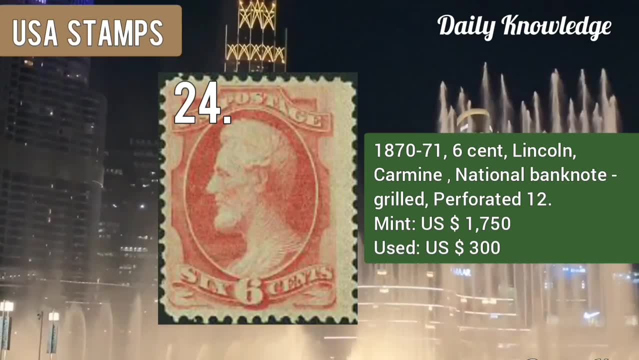 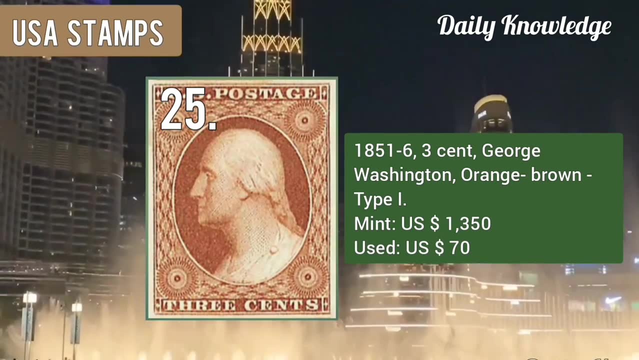 1869, 15 cent. columbus type 1 pictorial issue, grilled and mint and juiced values. 1870 to 71, 6 cent. lincoln carmine national banknote. it is grilled and perforated. 12, 1851 to 56, 3 cent. 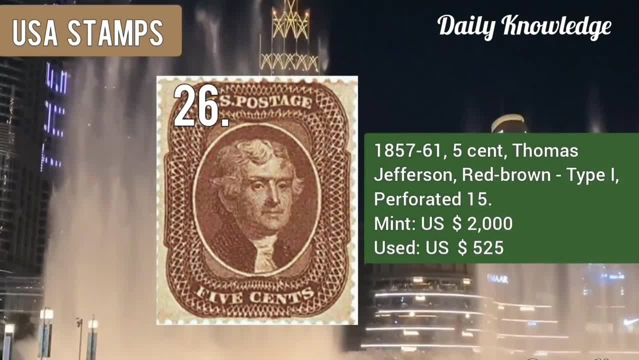 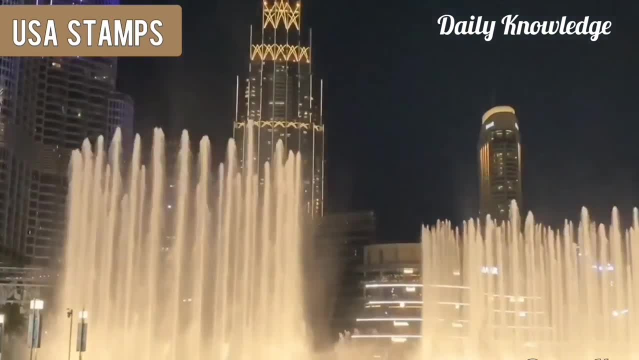 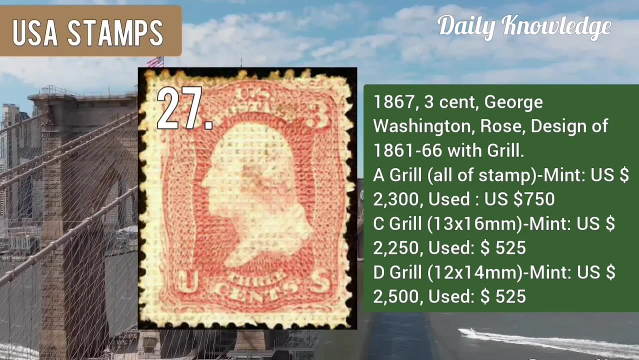 george washington, orange, brown and type 1, 1857 to 61, 5 cent. thomas jefferson, it is red, brown, type 1 and perforated 15, 1867, 3 cent. george washington, rose and design of 1861 to 66 with grill, 1870 to. 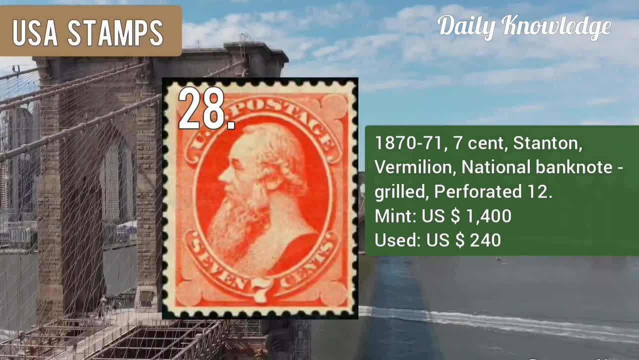 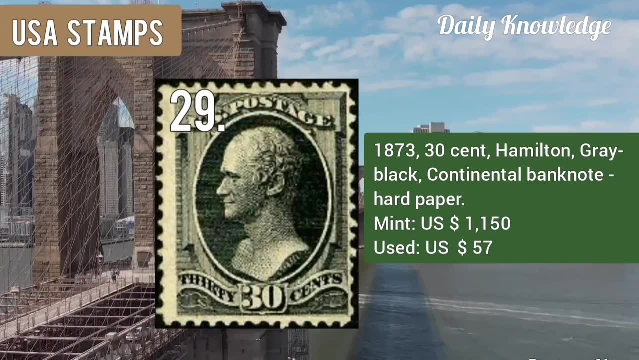 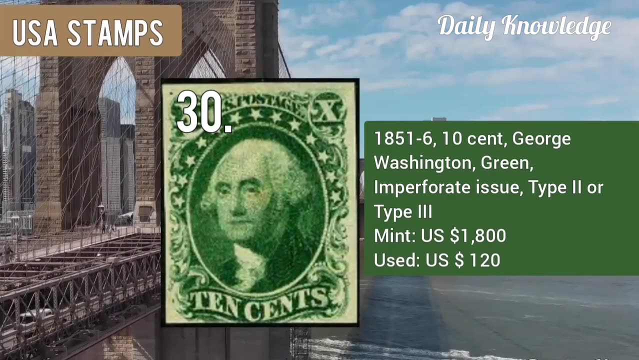 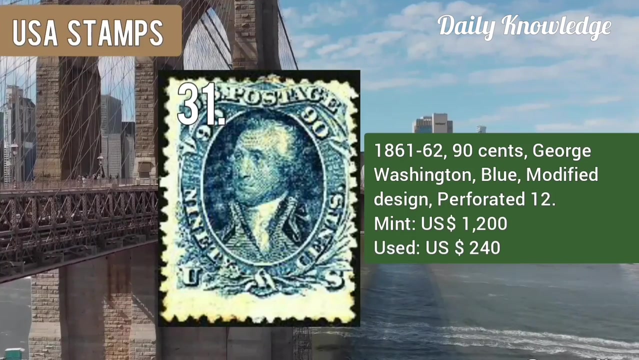 71, 7 cent stanton vermilion national banknote, grilled issue- 1873. 30 cent hamilton gray black color continental banknote, company issue on hard paper. 1851 to 56, 10 cent george washington green in perforate issue type 2 or type 3 values. 1861 to 62, 90 cent george washington blue. 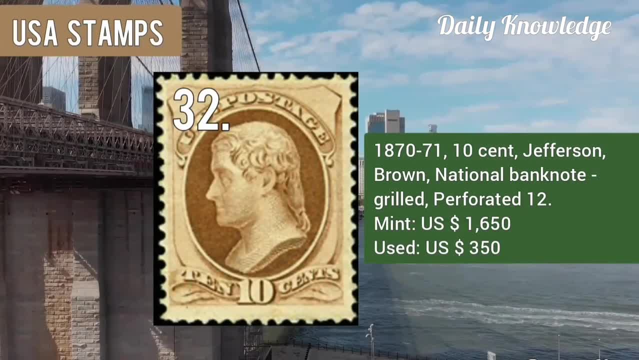 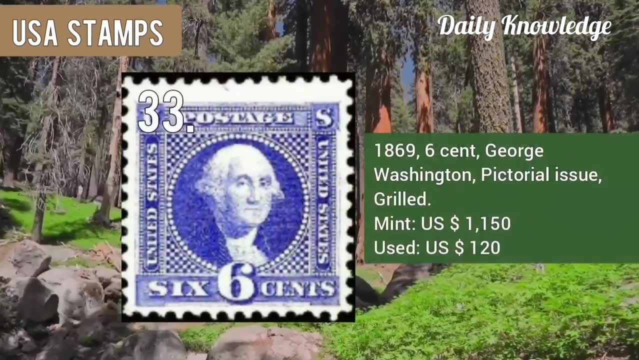 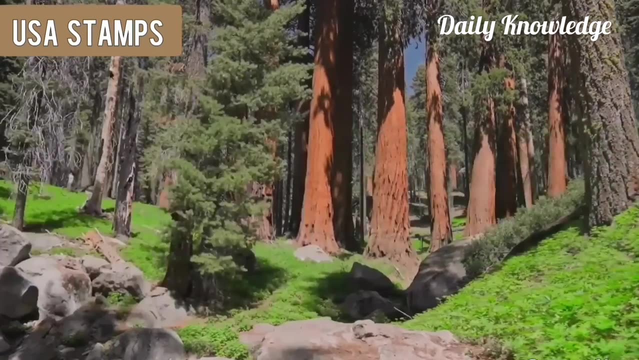 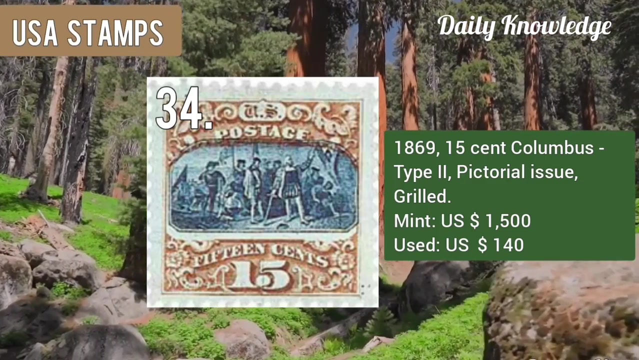 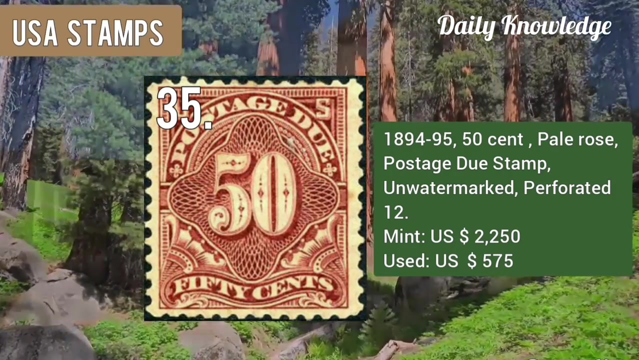 modified design and perforation: 12, 1870 to 71, 10 cent jefferson brown national banknote, grilled issue perforated. 12 1869, 6 cent george washington pictorial issue and grilled. next is 15 cent columbus type 2 pictorial issue and it is grilled. this is 1894 to 95, 50 cent pale rose. 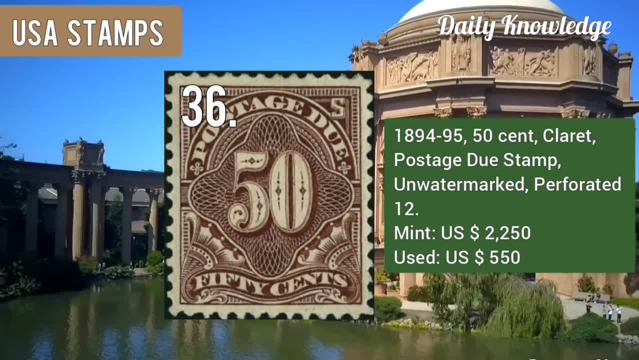 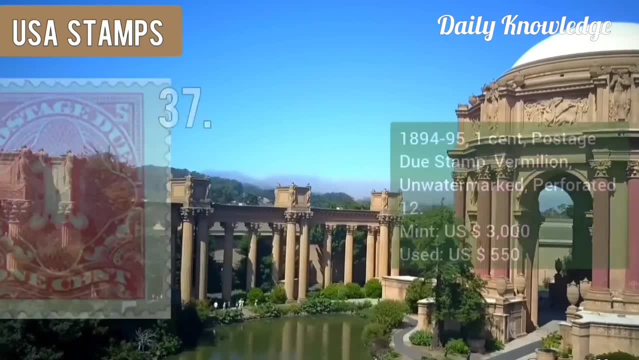 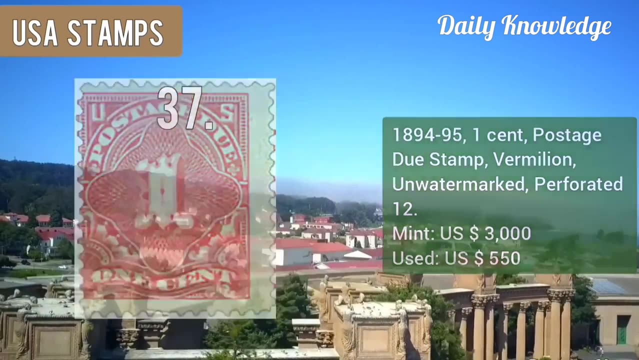 postage 2 stamp. it is unwatermarked and perforated. 1894 to 95 50 cent. claret postage 2 stamp, unwatermarked and perforated. 12. 1894 to 95 1 cent. postage 2 vermilion, unwatermarked and perforation. 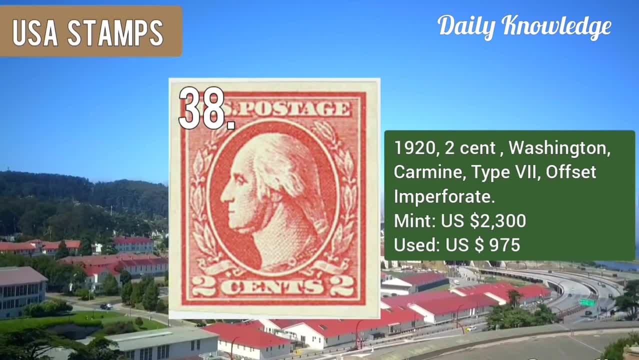 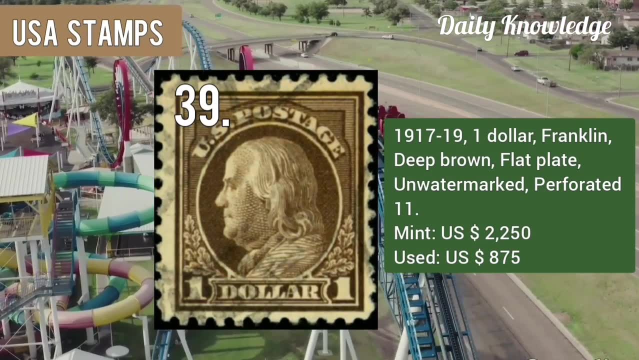 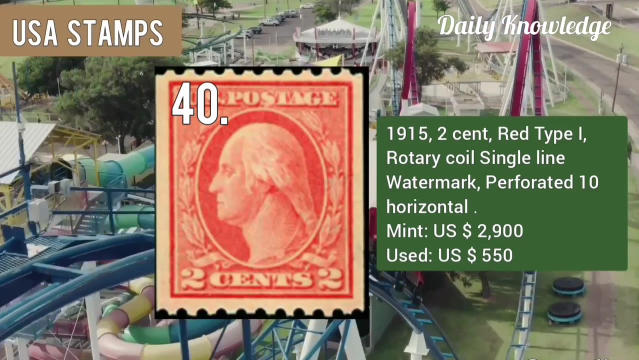 1922 2 cent washington carmine type 7 offset lithography and it is in perforate. 1917 to 19 1 dollar franklin deep, brown flat plate, unwatermarked and perforation 11. then 1915 2 cent red type 1 rotary coil single line, watermarked, perforation 10 and horizontal. 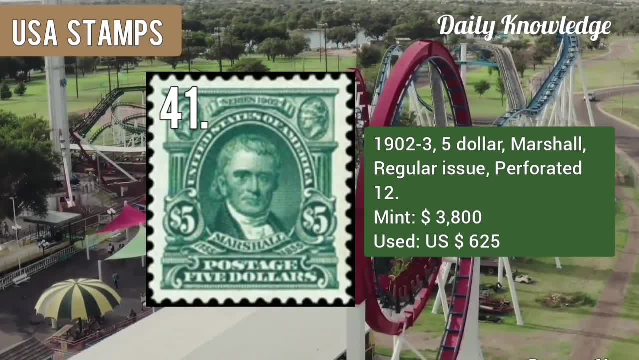 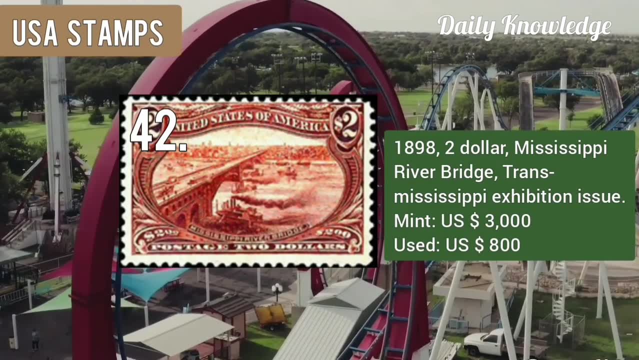 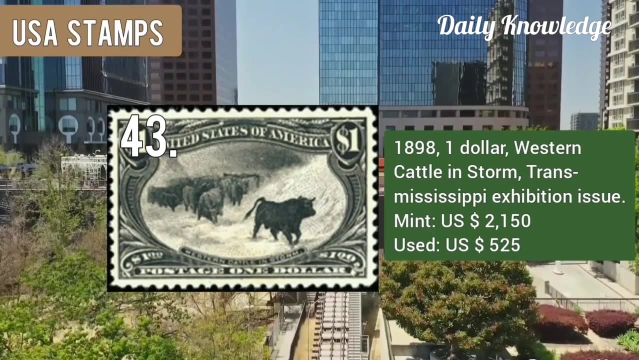 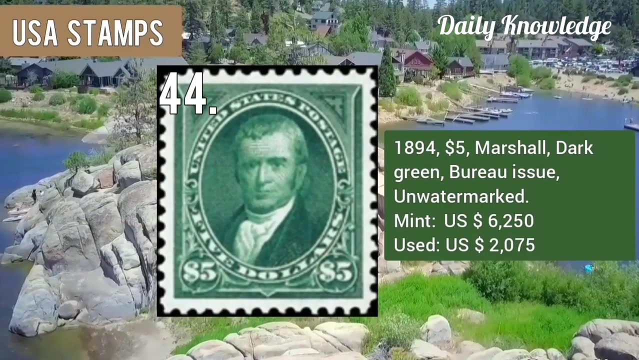 1902 to 3. five dollar marshall regular issue, perforated 12.. this is 1898. two dollar mississippi river bridge, trans-mississippi exhibition issue. now, this is 1898. one dollar western cattle in strong, trans-mississippi exhibition issue. this is 1894. five dollar marshall dark green bureau issue. 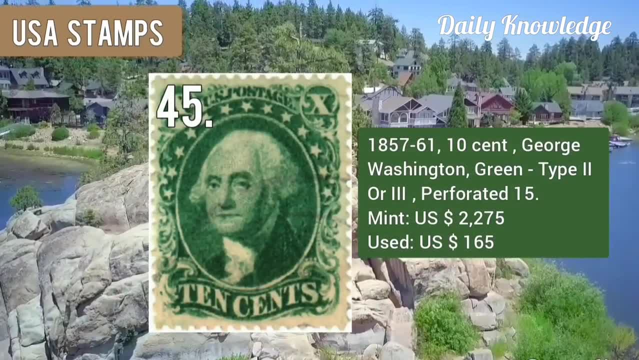 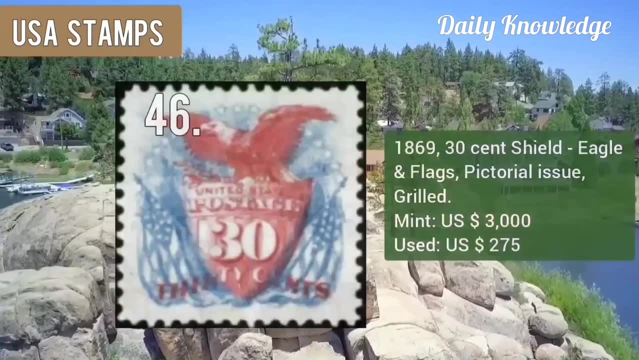 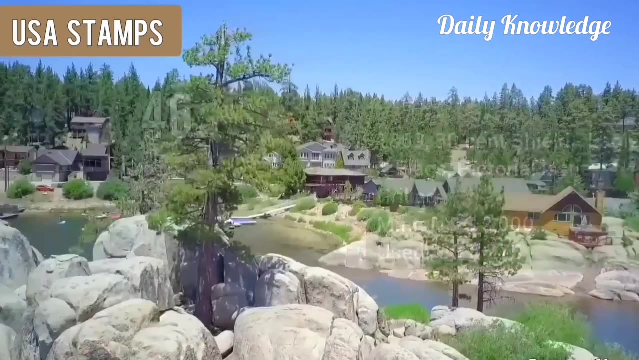 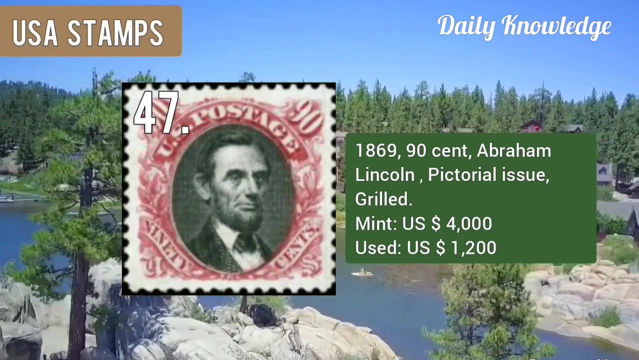 unwatermarked mint and used values. 1857 to 61, 10 cent george washington green color, type 2 or type 3 and perforated. 1869, 30 cent shield, eagle and flex pictorial issue and it is grilled. 1869, 90 cent abraham lincoln pictorial issue and it is grilled. wind and used values. 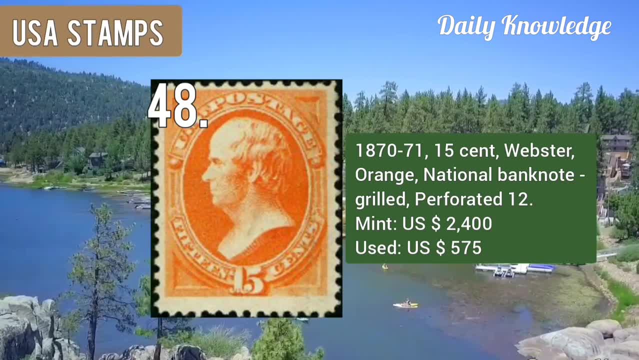 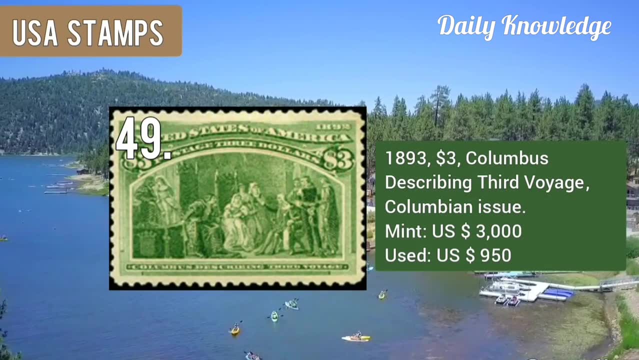 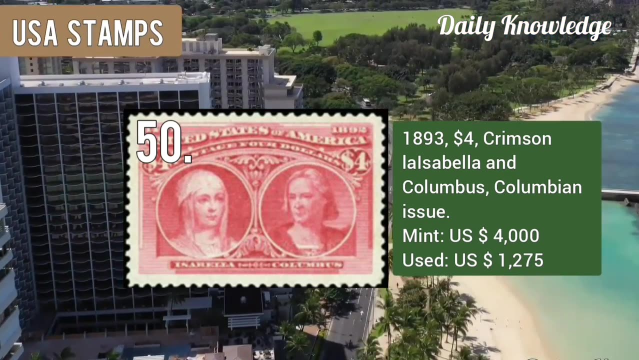 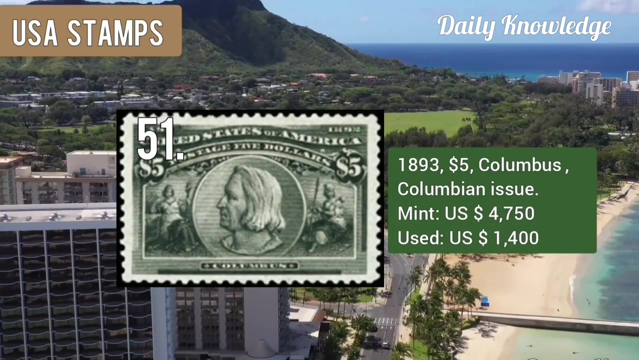 1870 to 71, 15 cent webster orange color national banknote, grilled and perforated. 1893, three dollar columbus describing third white columbian issue mint and used values. 1893, four dollar crimson isabella and columbus columbian issue mint and used values. 1893, 5 columbus columbian issue mint and used values. 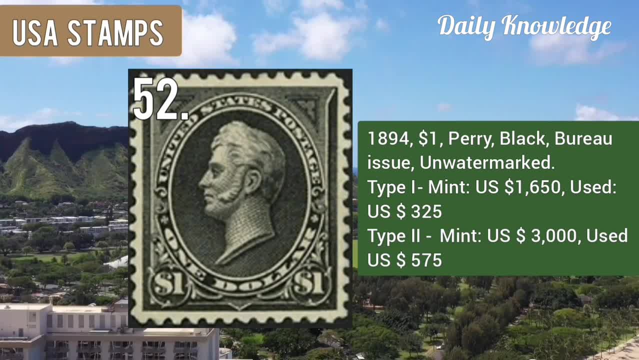 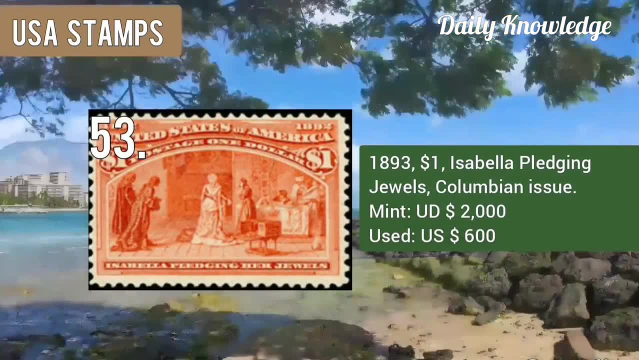 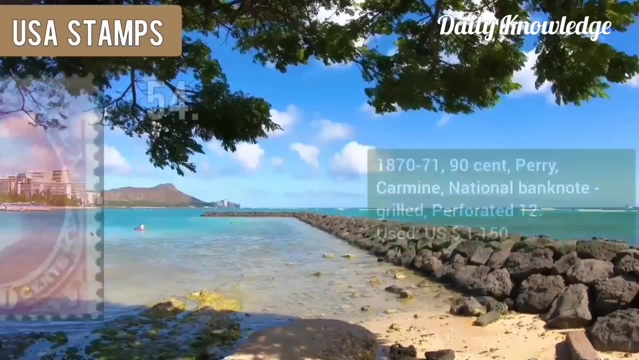 are given next is 1894: one dollar. very black bureau issue, unwatermarked type 1 mint and juiced values. 1893: one dollar. isabella pledging jews. colombian issue, mint and used values. 1870 to 71: 90 cent. pericaraha national banknote grill. 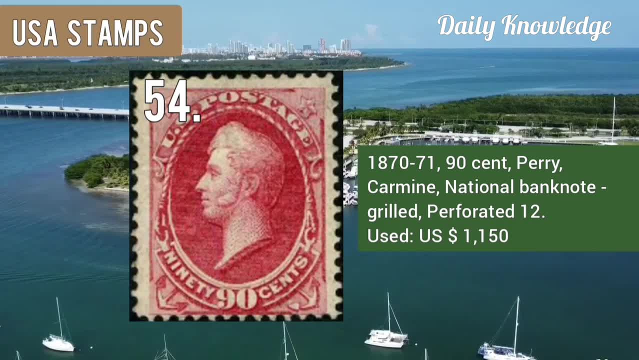 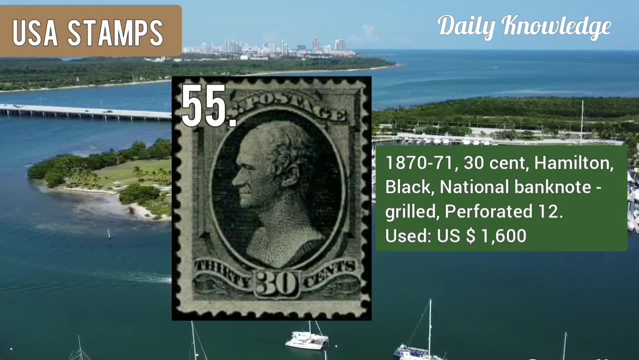 tissue with perforation 12.. 1870 to 71, 30 cent hamilton black national banknote grill tissue perforated. probably three dollarimizi hundred and fifty ten hundred neces. chris ievichaskadivin, sp. hulbos patashi. 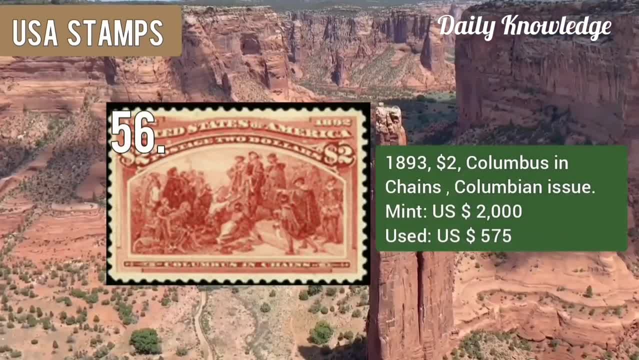 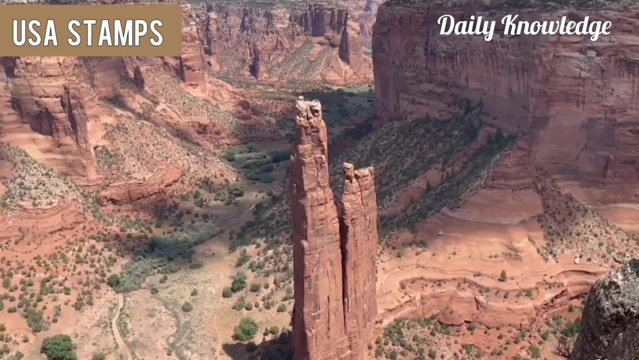 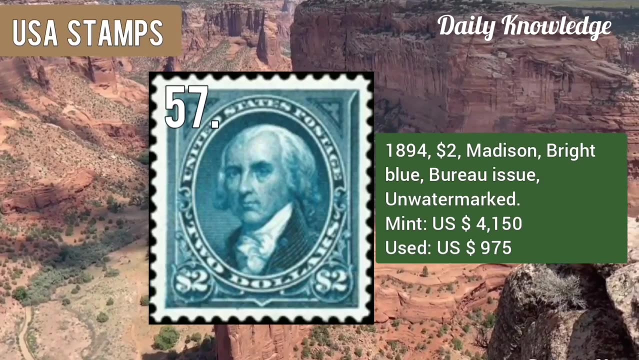 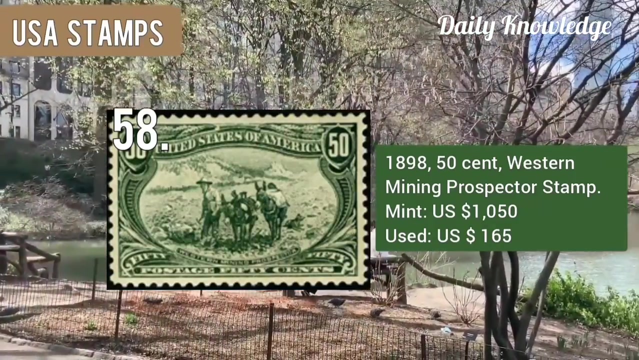 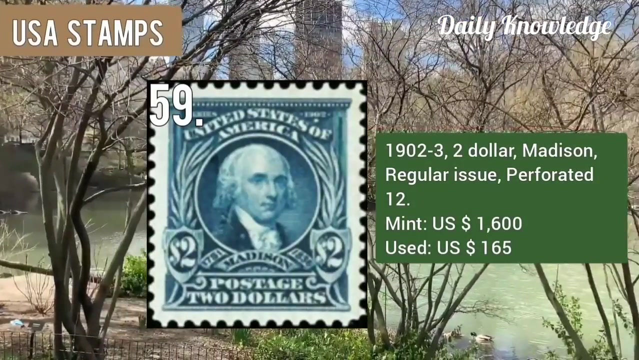 um cl. angel tel Zhao, operation 12. next is 1893: two dollar columbus in chains columbian issue, mint and used values. now, 1894, two dollar medicine, bright blue bureau issue, unwatermarked. next is 1898, 50 cent western mining prospector stamp- it is mint and used values. 1902 to three: two dollar medicine, regular. 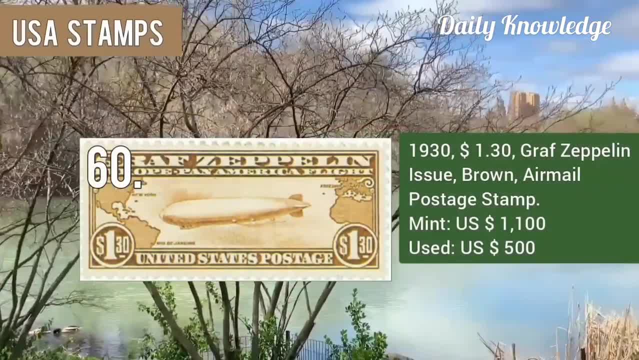 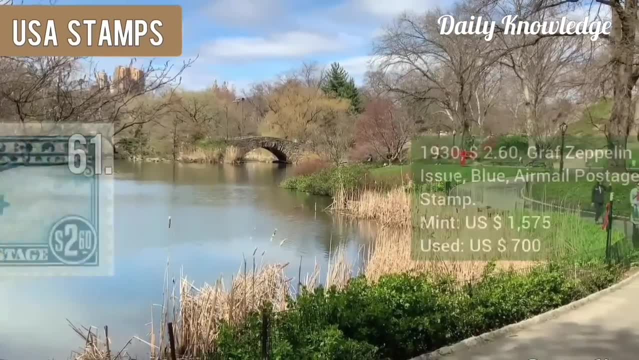 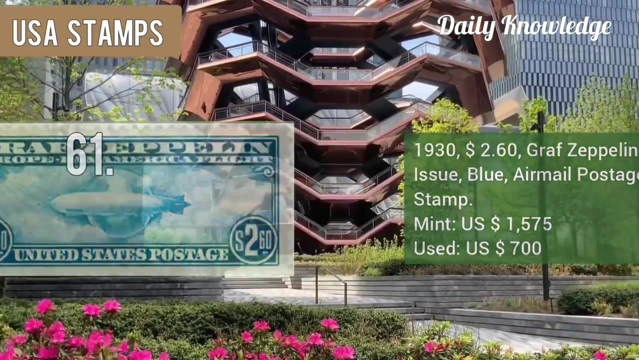 issue: perforation 12 and mint and used values: 1930: 1.30 dollar. graph- zeppelin- brown color air mill stamp. 1930: 2.60 dollar. graph- zeppelin- blue color air mill postage stamp. next is 1903: two dollar medicine regular issue: perforation 12 and mint and used values: 1903: two dollar. 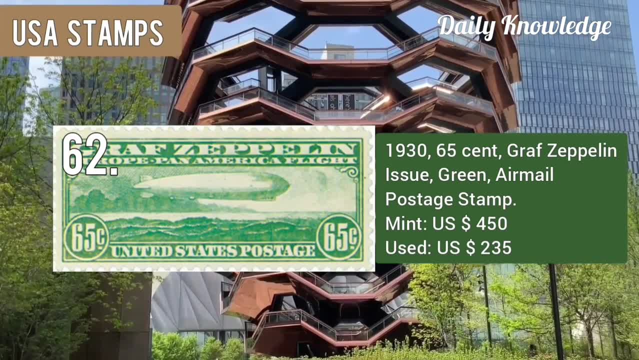 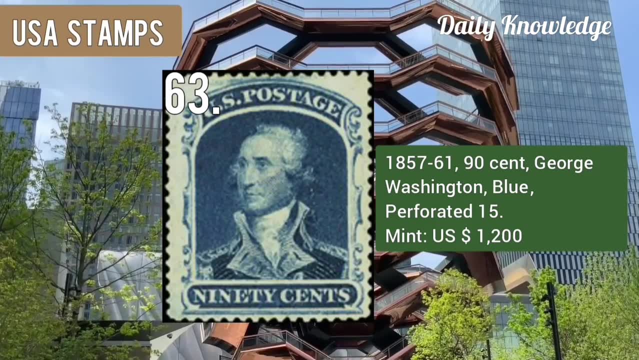 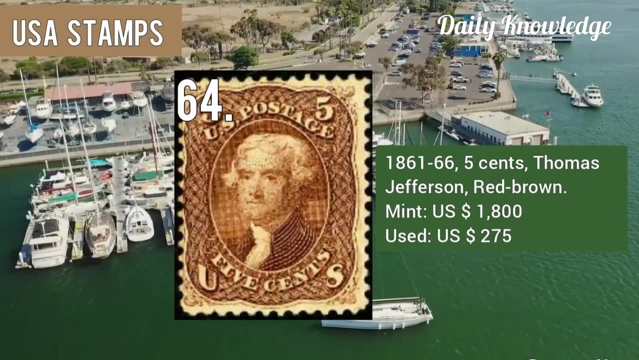 1830, 65 cent Kraft Zeppelin and it is green color. air mill postage stamp. 1857 to 61,, 90 cent George Washington: blue color and perforation 15.. 1861 to 66,, 5 cent Thomas Jefferson: red, brown color. 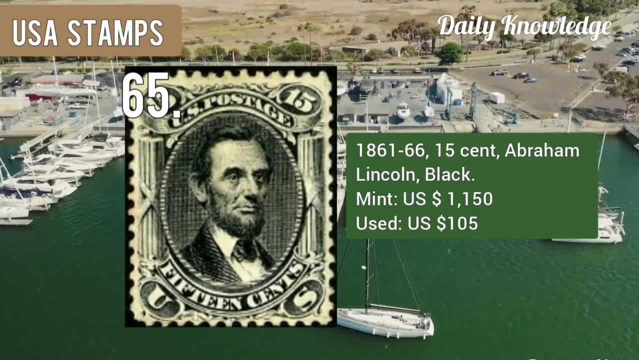 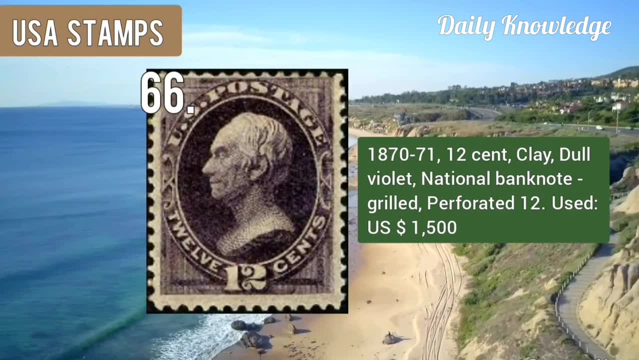 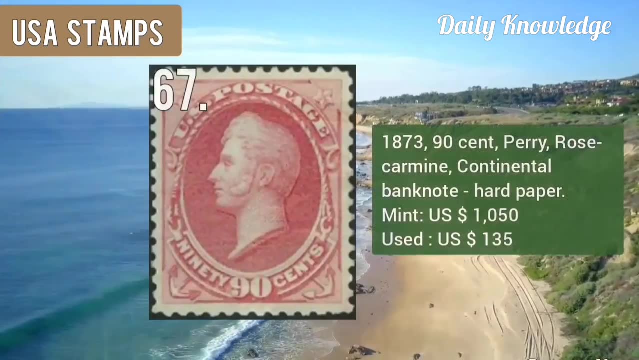 Next is 1861 to 66, 15 cent Abraham Lincoln black color stamp and mint-induced values. Now 1870 to 71,, 12 cent clay dull violet color national banknote, grill tissue. 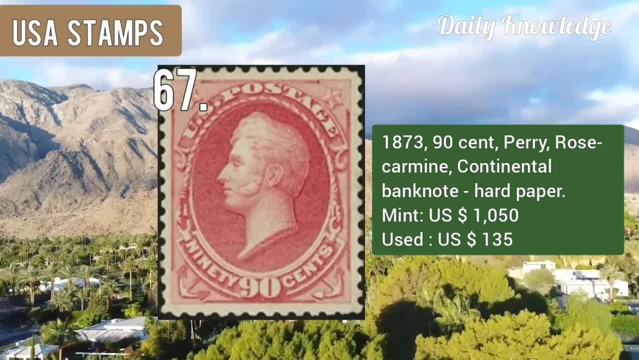 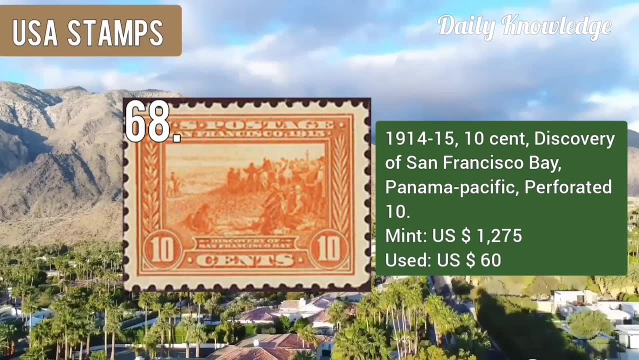 1873, 90 cent Perry rose carmine continental banknote and it is hard paper. 1914 to 15, 10 cent. Discovery of St Francisco Bay, Panama Pacific perforation 10.. 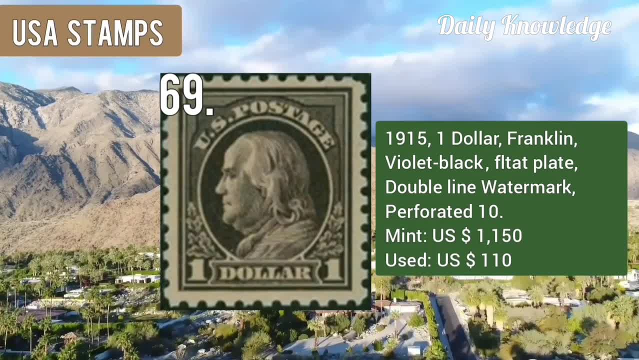 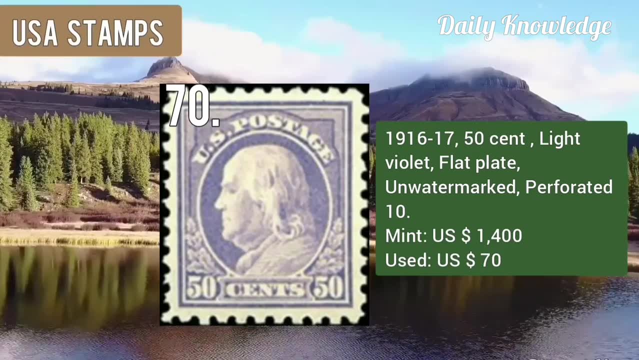 1915, $1, Franklin violet black first plate and double line, watermarked and perforation 10.. 1916 to 17, 50 cent light violet flat plate, un-watermarked and perforation 10.. 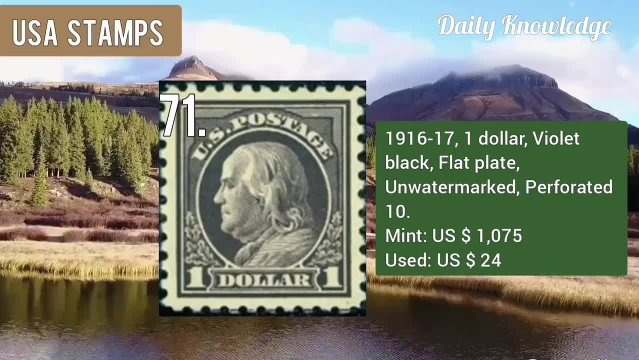 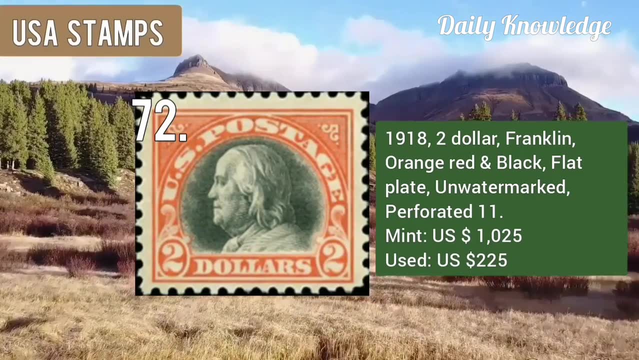 This is 1916 to 17,. $1, violet- black flat plate, un-watermarked and perforation 10.. 1918.. $2, Franklin, orange, red and black flat plate, un-watermarked and perforation 11.. 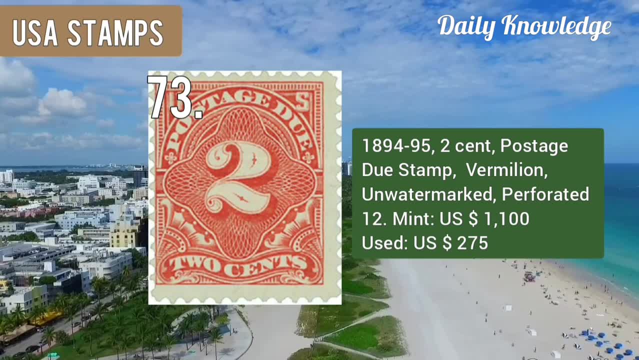 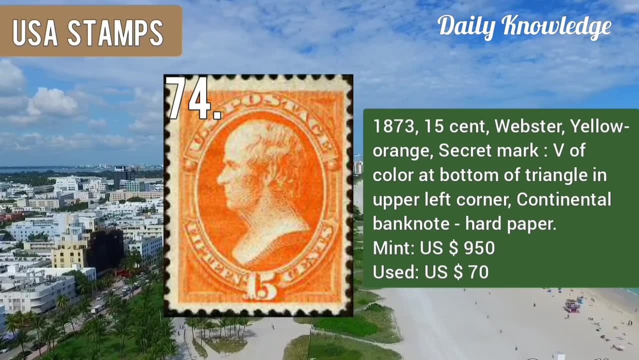 1894 to 95, 2 cent postage due stamp, vermilion, un-watermarked, and perforation. 12. 1873, 15 cent Webster yellow-orange with cigarette mark V of the color at bottom of triangle in the upper left corner. 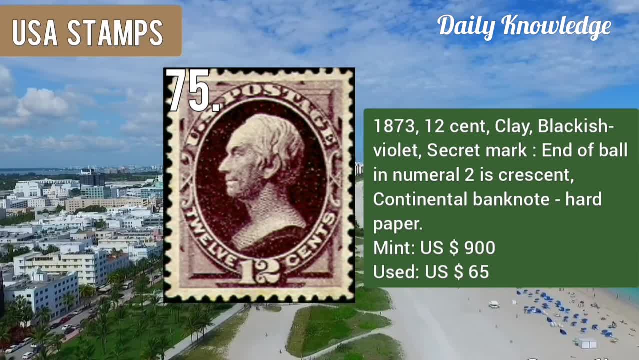 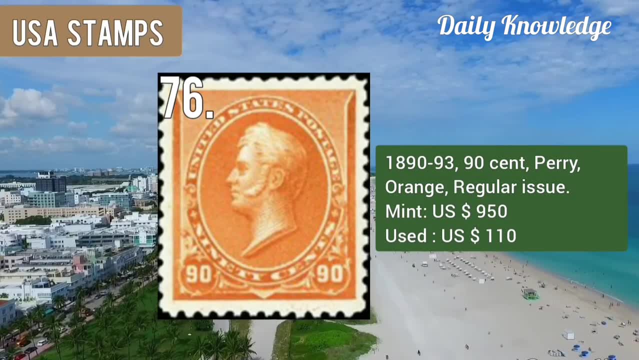 1873, 12 cent clay blackish violet with cigarette mark and it is a continental banknote on hard paper. 1890 to 93, 90 cent peri-orange color regular issue, mint-induced values. 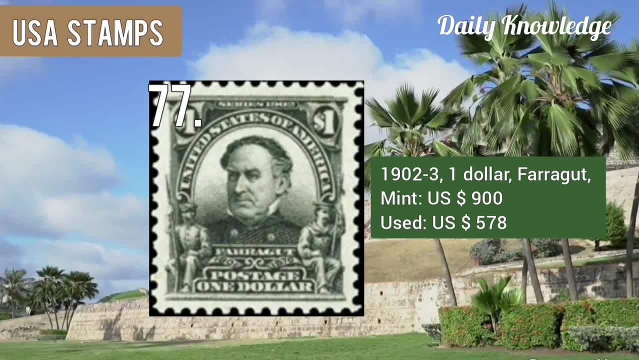 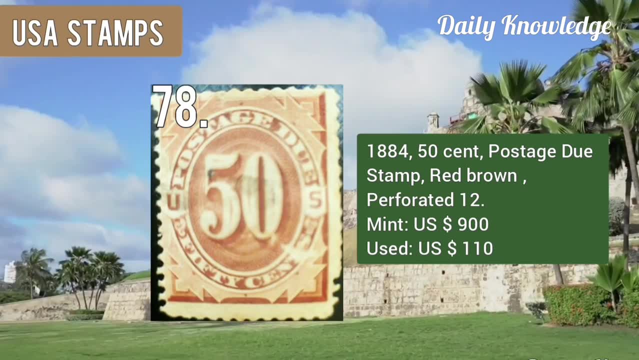 1902 to 1903, $1, Farragut issue mint-induced values 1884,. 50 cent postage due stamp, red-brown color and perforation. 12.. 1857 to 61, 30 cent Benjamin Franklin: orange color and perforation. 12.. 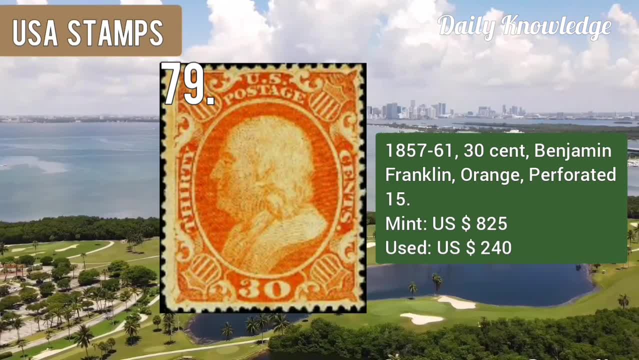 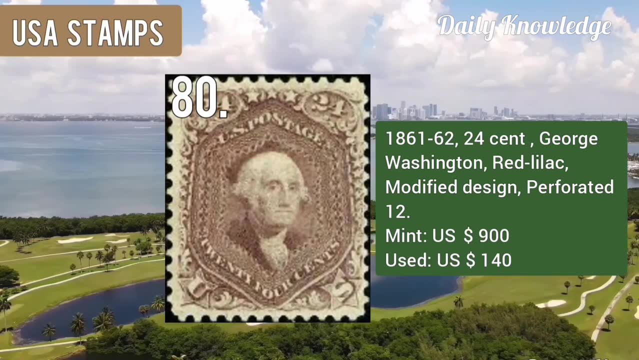 Now this is 1857 to 61,, 30 cent Benjamin Franklin: orange color and perforation. 12.. 1861 to 62,, 24 cent George Washington: red liliac modified design and perforation. 12.. 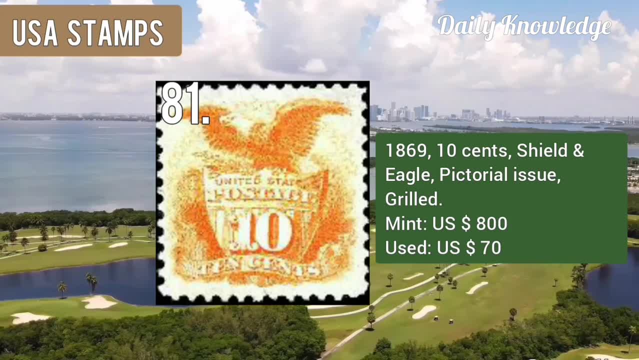 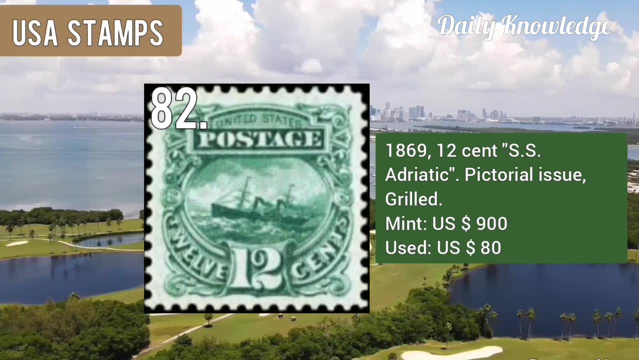 1869, 10 cent Shield and Eagle pictorial issue, and it is grailed. Next is 1869, 12 cent SS Adriatic pictorial issue, and it is also grailed. 1870 to 71, 116.. 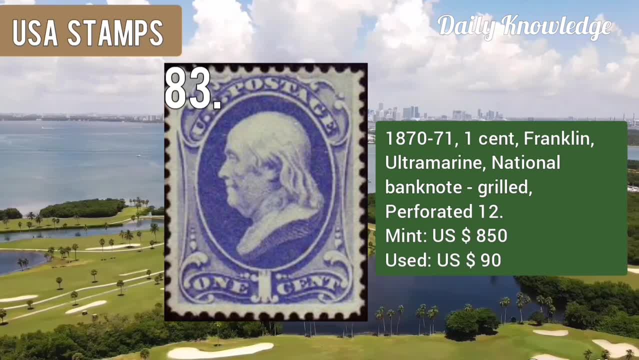 1871 to 71,. 1 cent George Washington, red-lighted modified design and perforation: 12.. 1881, 1 cent franklin, ultramarine national banknote, creel, tissue perforation- 12. now this is 1881 to. 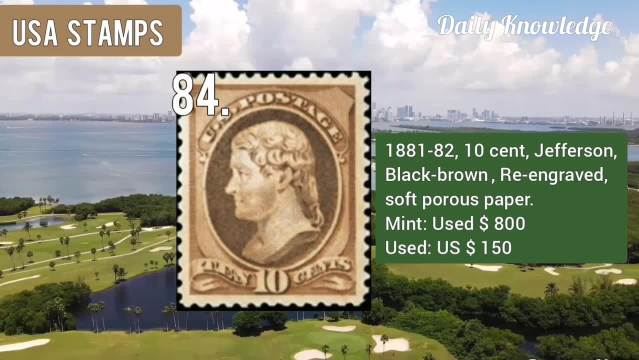 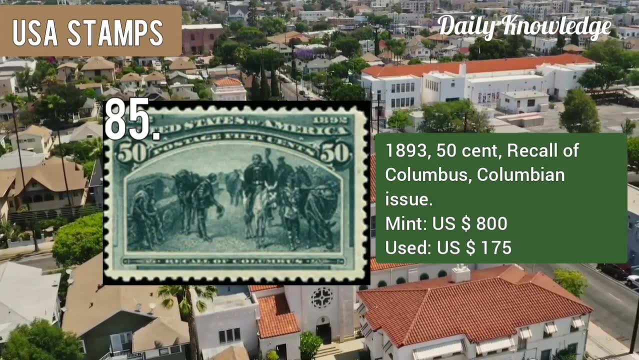 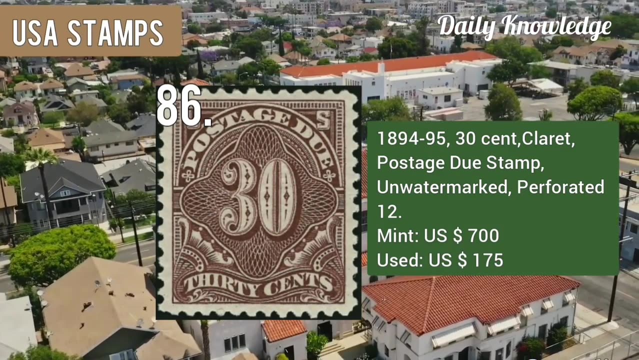 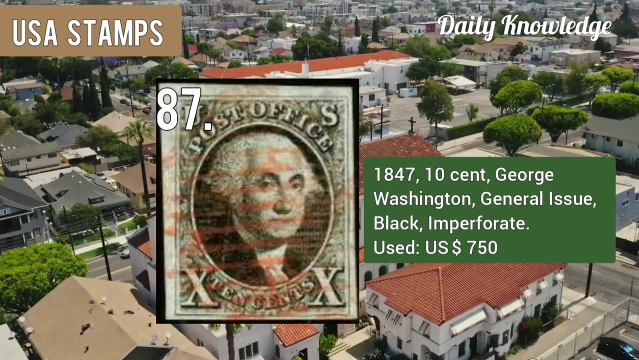 82 10 cent jefferson, black, brown, re-engraved on soft porous paper. 1893, 50 cent. recall of the columbus columbian issue, mint and used values. 1894 to 95, 30 cent claret postage due stamp. it is unwatermarked and perforated. 1847 10 cent george washington general issue: black color. 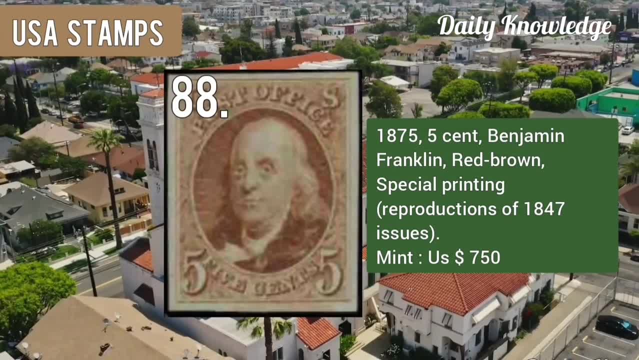 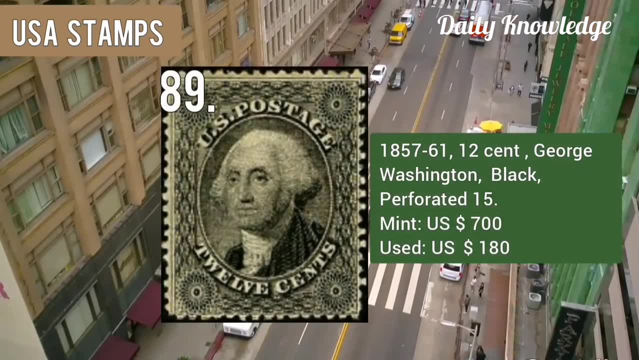 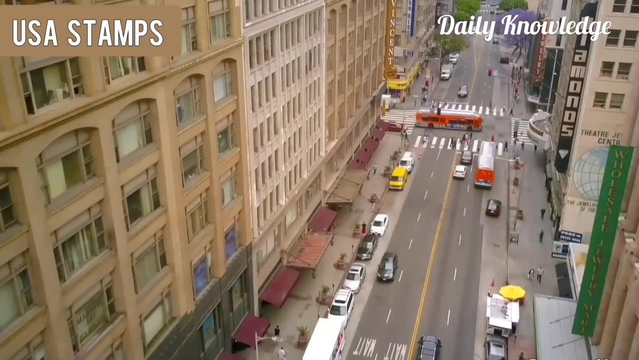 and in perforate now: 1875, 5 cent. benjamin franklin, red, brown, special printing reproduction of 1847 issue. 1857 to 61, 12 cent, george washington, black color, and it is perforated 15, 1861 to 62, 12 cent. 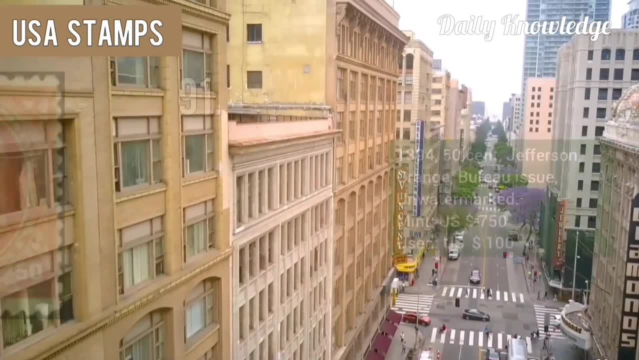 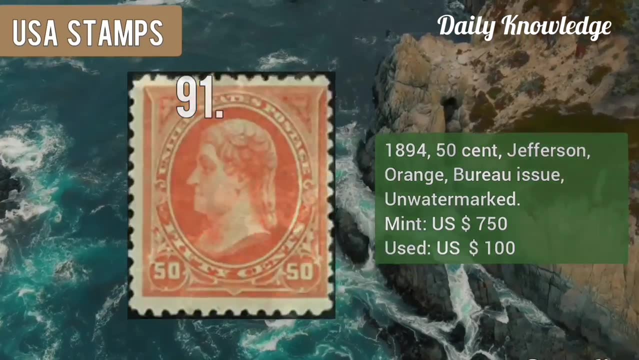 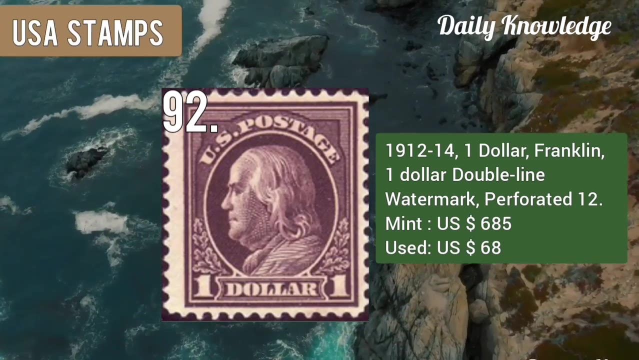 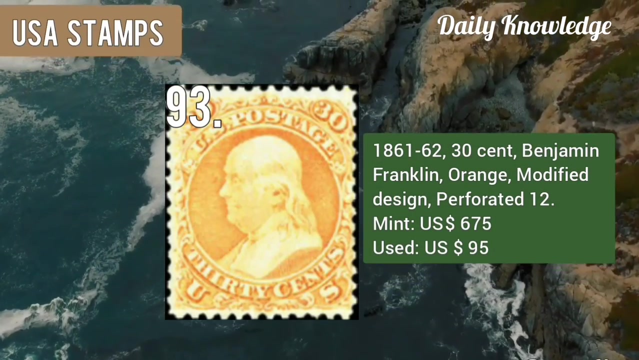 george washington, black color, modified design and perforated. now 1894. 50 cent jefferson, orange, color, bureau issue, unwatermarked. now this is 1912 to 1914. one dollar franklin, one dollar double line and perforation. 12, 1861 to 62, 30 cent benjamin franklin, orange color, modified design and. 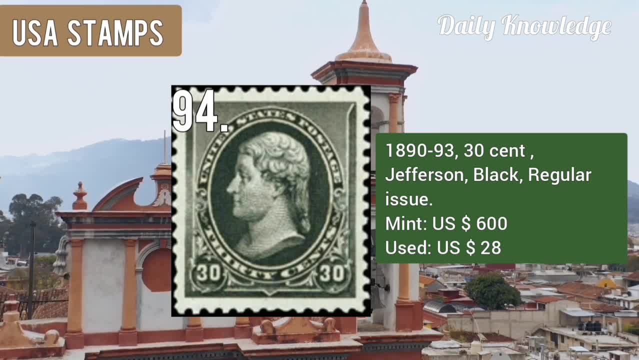 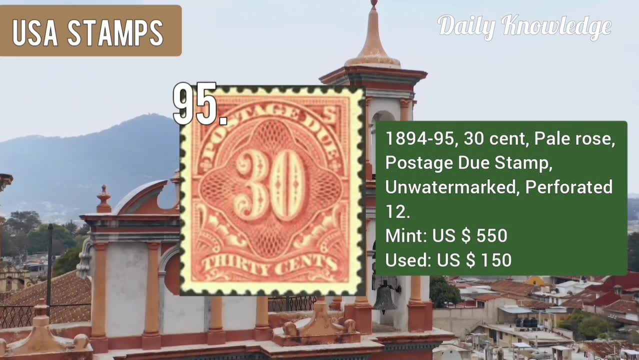 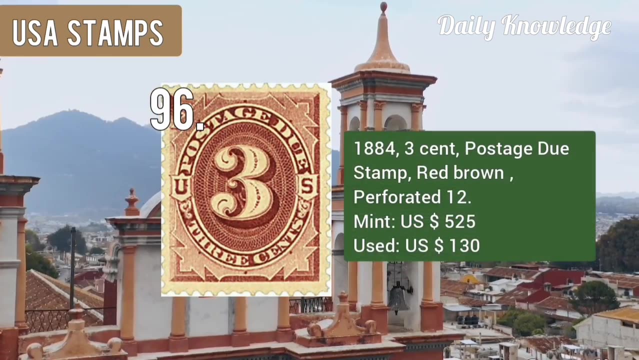 perforation 12, 1891 to 93, 30 cent jefferson black color stamp and it is a regular issue. next is 1894 to 95, 30 cent pale rose postage 2 stamp, unwatermarked, and perforation 12, 1884, 3 cent postage 2 stamp. 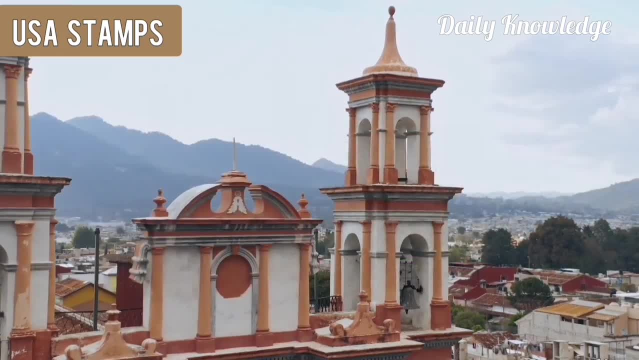 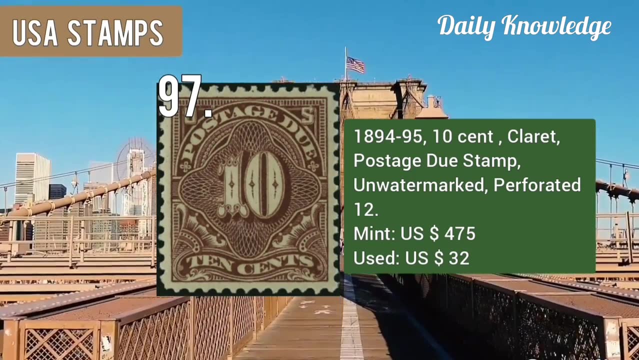 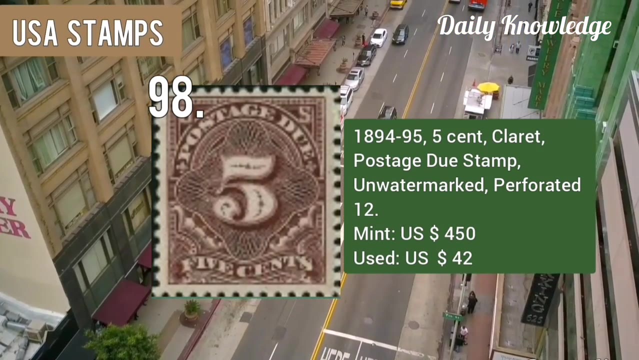 red, brown color and perforated 12. now this is 1894 to 95, 10 cent claret postage 2 stamp, unwatermarked and perforated 12. 1894 to 95, 5 cent claret postage 2 stamp, unwatermarked and. 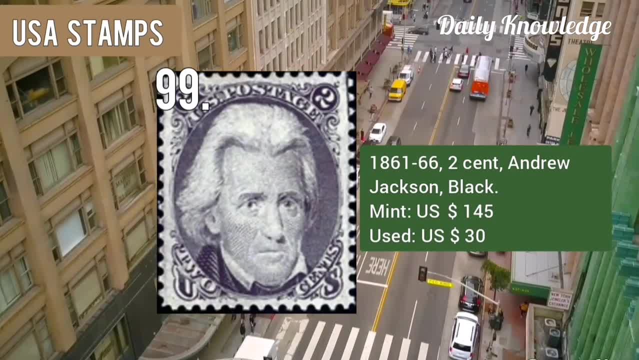 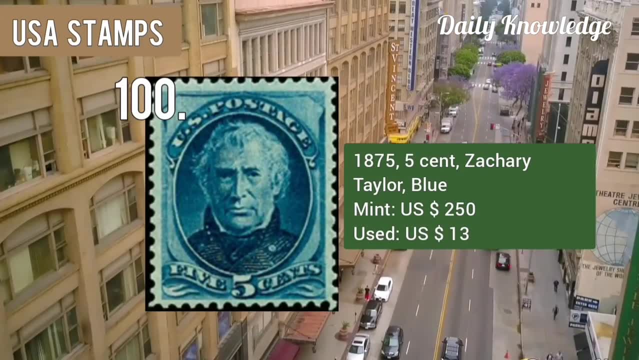 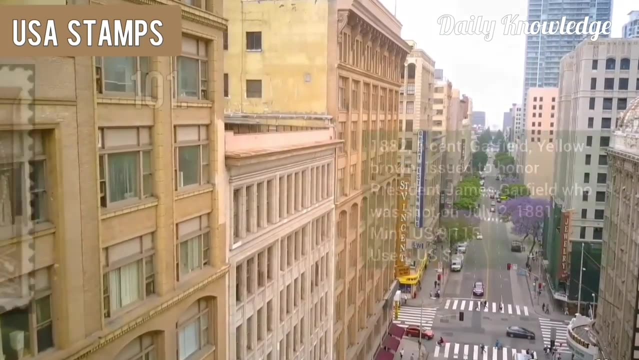 perforated 12, 1861 to 66, 2 cent. entreo jackson black color stamp and mint and used values. now 1875, 5 cent. taylor blue color stamp, mint and used values are given here. next is 1882, 5 cent. 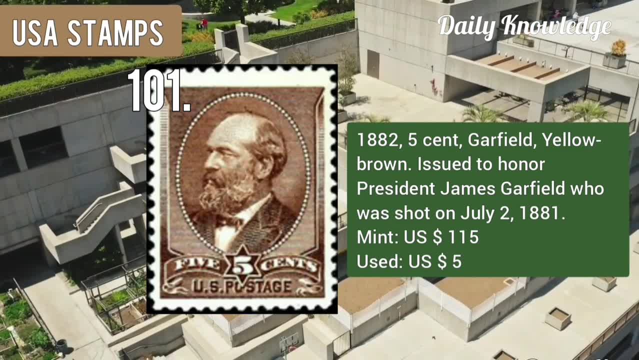 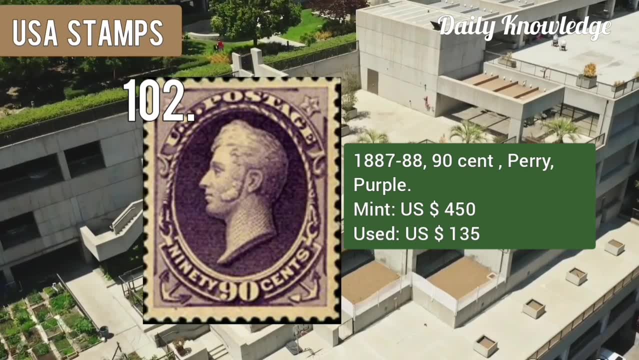 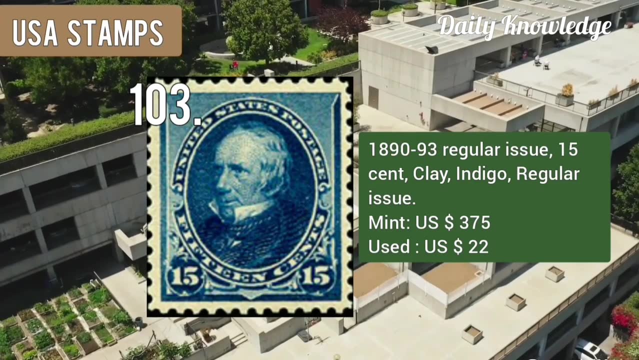 garfield garfield, garfield yellow brown issued to honor president james garfield. now 1887 to 88, 90 cent. berry purple color stamp and the mint and the used values are given: 1890 to 93: regular issue: 15 cent. clay and indigo color: regular issue. next is 1898, 4 cent. 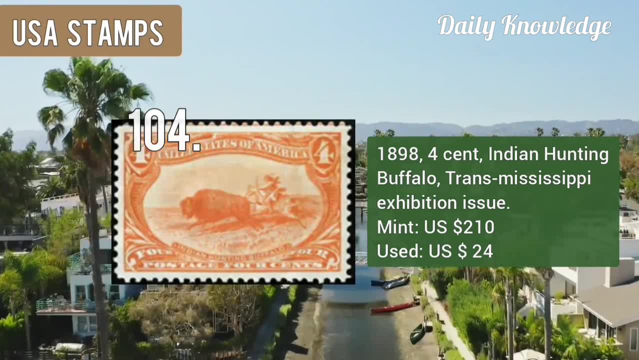 indian hunting buffalo- trans-mississippi exhibition issue. this stamp is from 1898. 4 cent indian hunting buffalo- trans-mississippi exhibition issue. this stamp is from 1898. 4 cent indian hunting buffalo- trans-mississippi exhibition issue. this stamp is from. 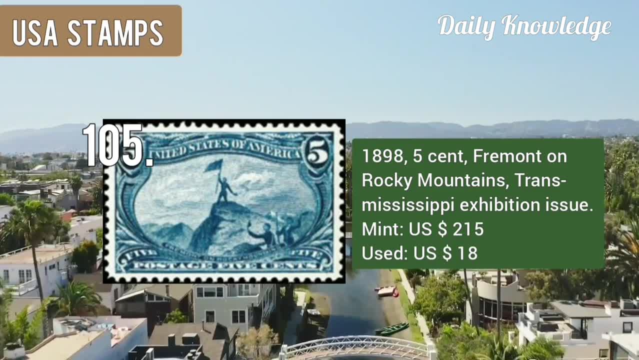 1898, 4 cent indian hunting buffalo- trans-mississippi exhibitioning issue 11 to 188, 5 cent fremont on rocky. 1898, 4 cent indian hunting buffalo- trans-mississippi exhibition issue 11 to 189, 5 cent fremont on rocky. 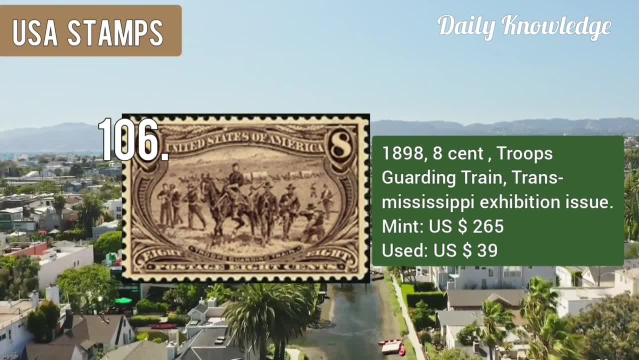 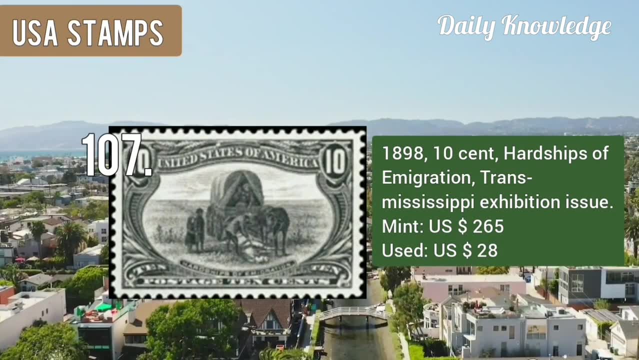 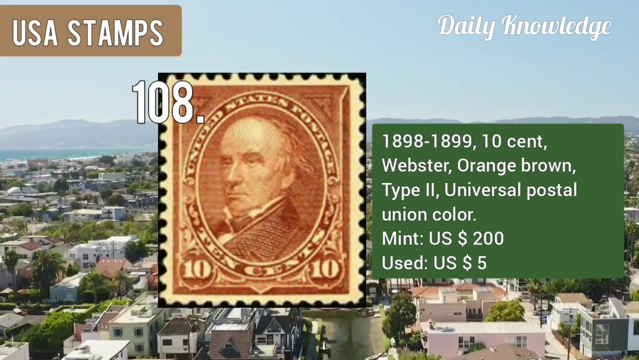 1898, 4 cent roll prairie tribal. 1898, 10 cent troop's garden train. transcripts is see the exhibition issue. 1898, 8 cent troops guarding train- USP. exhibition issue. next is next is next is 10, sometime next is it it nitrate 10 cent hard shapes of immigration. it is also transmit the logr城群��면 7个 отдolar印等和国国耕zych GIS MIS and it is also transcripts issue. 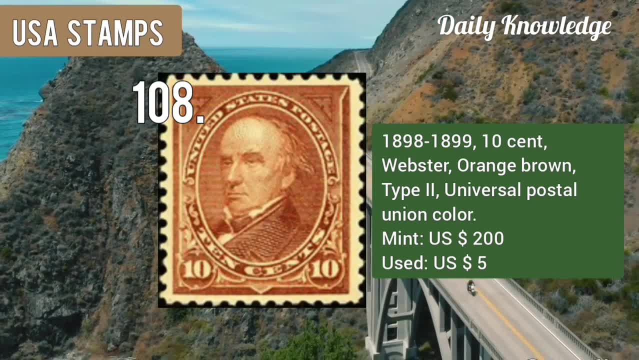 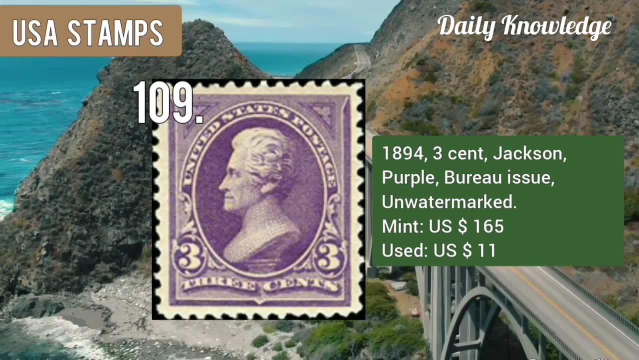 1898 8 są 1在去嘍 168, 189. Club closest to in is aæ 90. Это还在 gettin nine. nine ten cent bremsen Center. deliver des Webster orange, brown color type 2. this is 1894, 3 cent Jackson purple bureau. 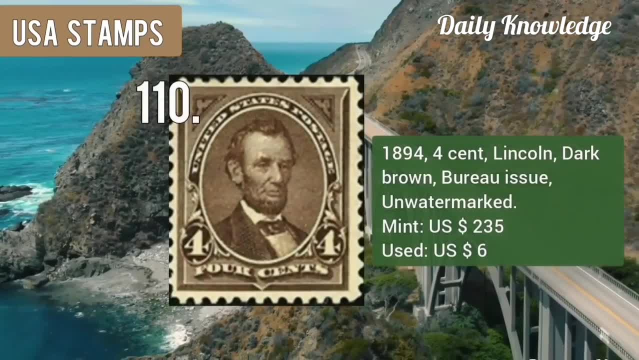 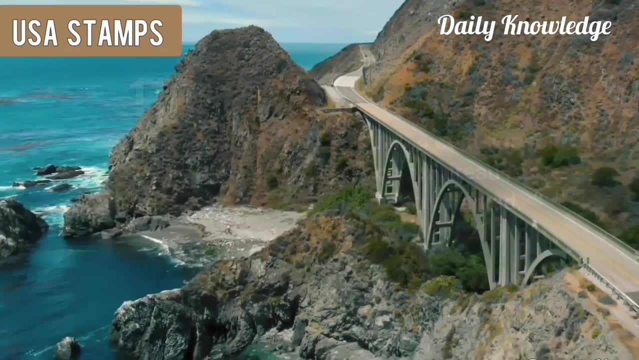 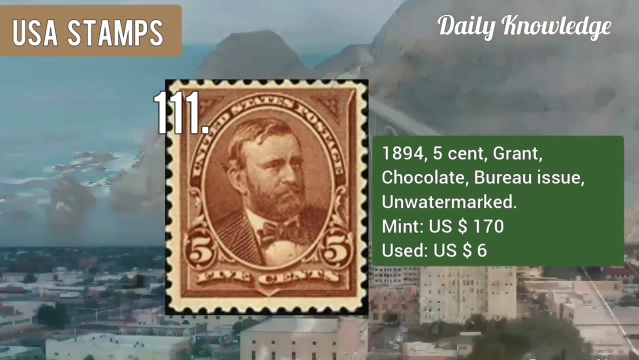 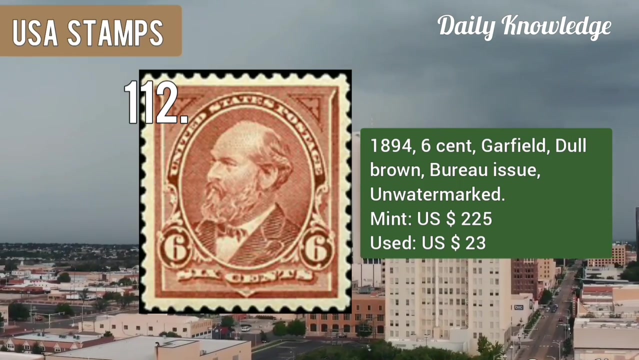 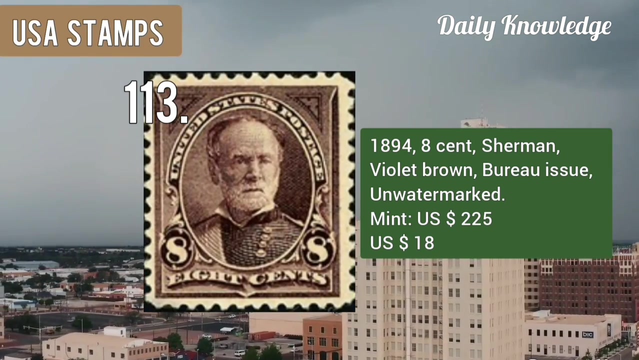 issue. now it is unwatermarked 1894, 4 cent Lincoln dark brown color bureau issue and it is also unwatermarked 1894, 5 cent Grant chocolate bureau issue, unwatermarked 1894, 6 cent car filledаш dual throwing bureau issue and it is also on Watermarked 1894. it's in Sherman. 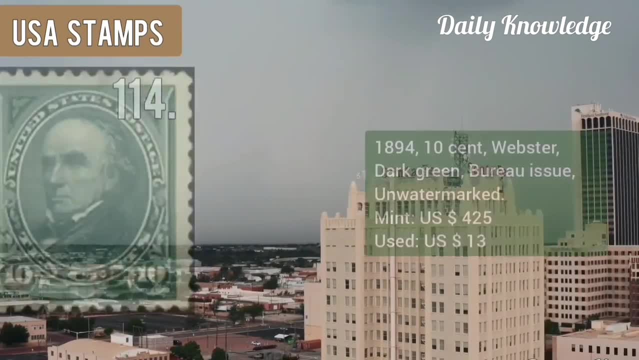 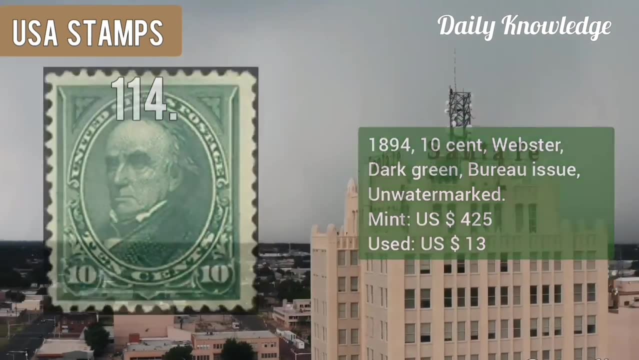 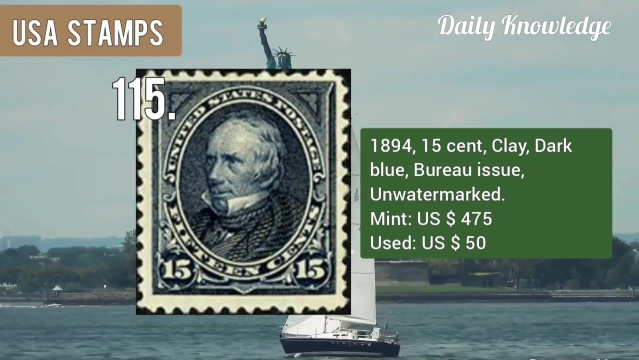 violet brown color bureau issue on Watermarked now 1894, ten cent. Webster dark green color bureau issue on Watermarked it is 94, 15 cent. Gley dark blue color bureau issue and underwater mark 1893, five cent soliciting aid from isabella colombian issue. 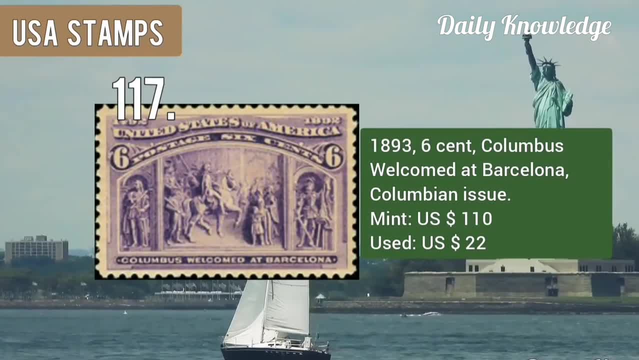 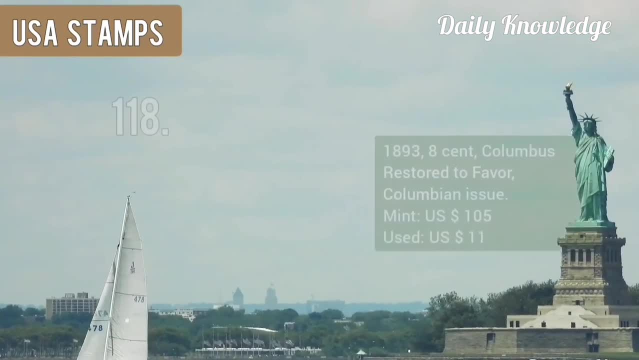 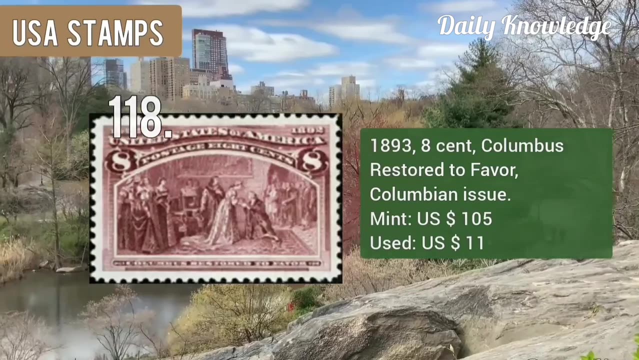 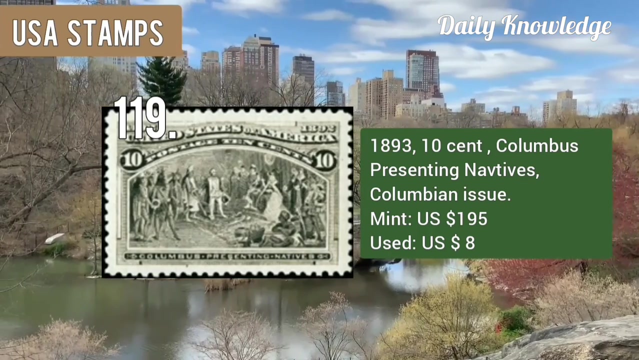 and maintain used values are given: 1893, six cent columbus welcomed at barcelona colombian issue and mint and used values. 1893, eight cent columbus, registered to favor colombian issue, mint and used values. 1893, 10 cent columbus presenting navities and it is a colombian issue. next is 1893, 15 cent. 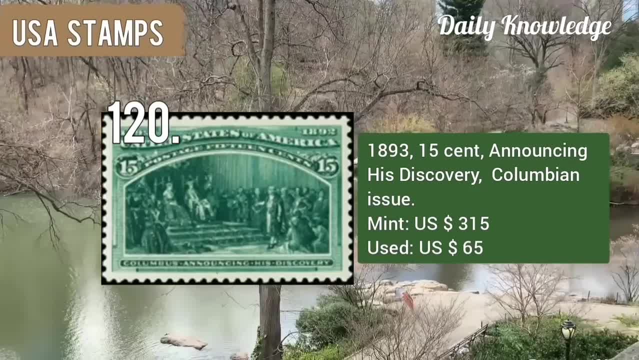 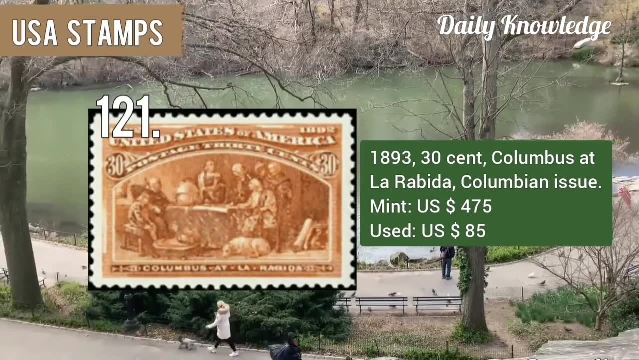 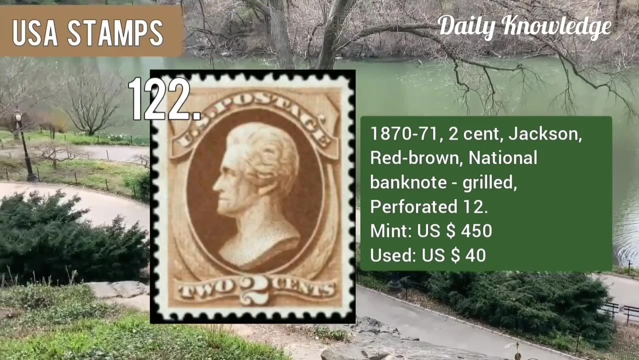 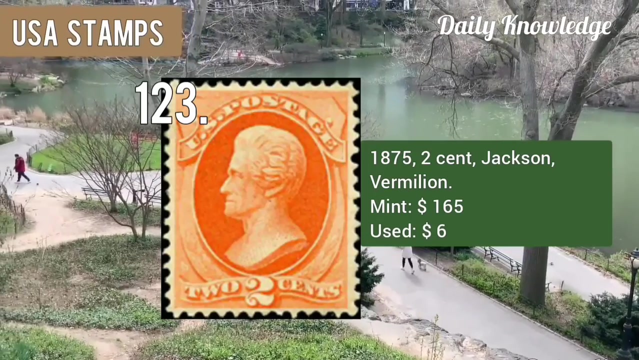 columbus announcing his discovery. colombian issue, perforated 1893, 30 cent columbus at la rabida. colombian issue, mint and used values 1870 to 71, 2 cent jackson red brown color national bank note grilled issue and perforated 12, 1875, 2 cent jackson vermillion. 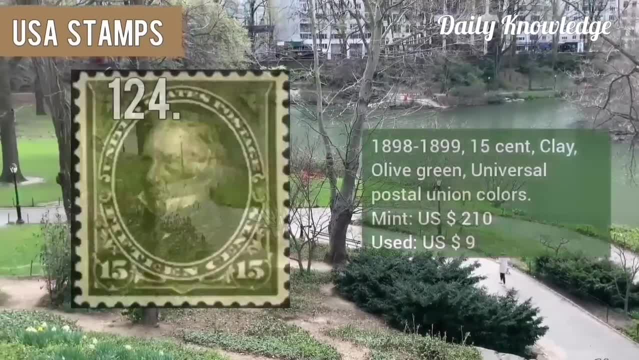 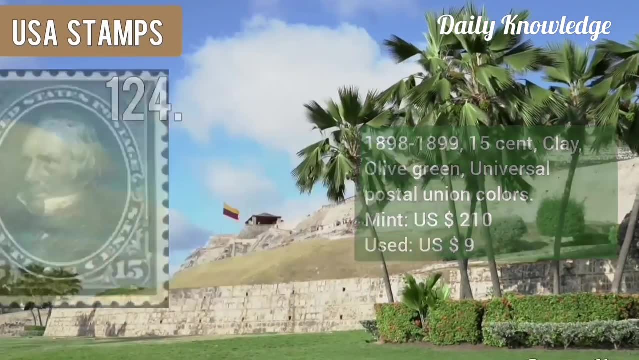 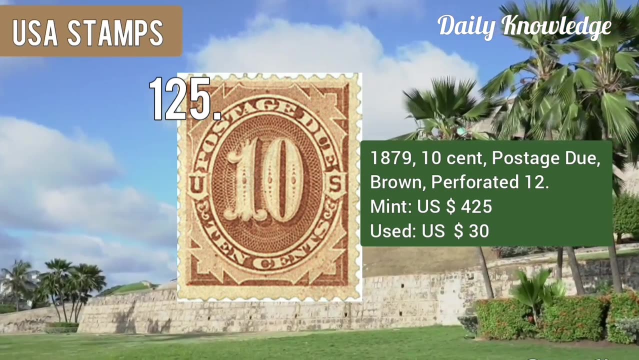 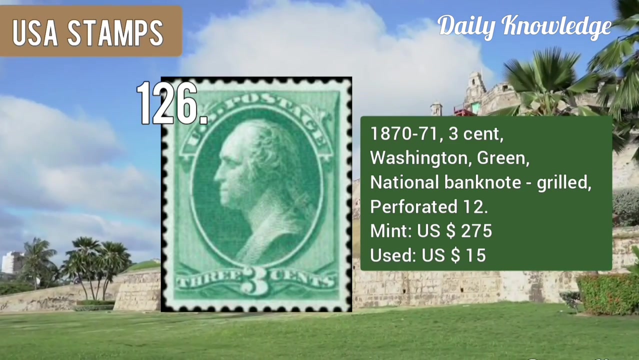 and mint and used values now: 1898 to 1899: 15 cent clay olive green color, universal postal union. 1879, 10 cent postage due brown color and perforated. 12 1870 to 71. three cent washington green color national banknote grill tissue. then 1851 to 56 one. 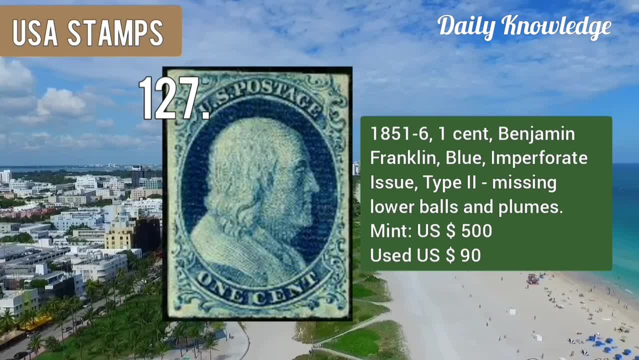 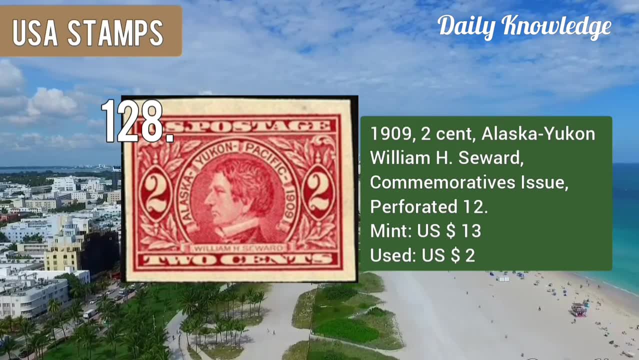 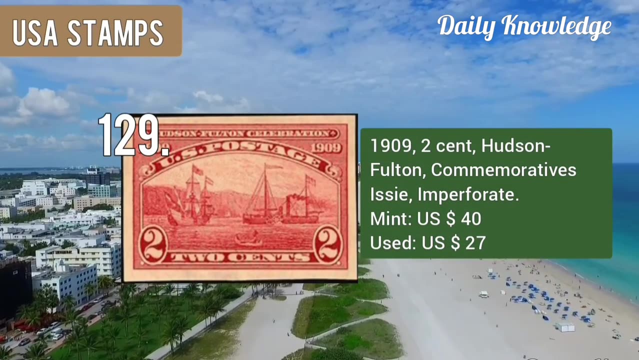 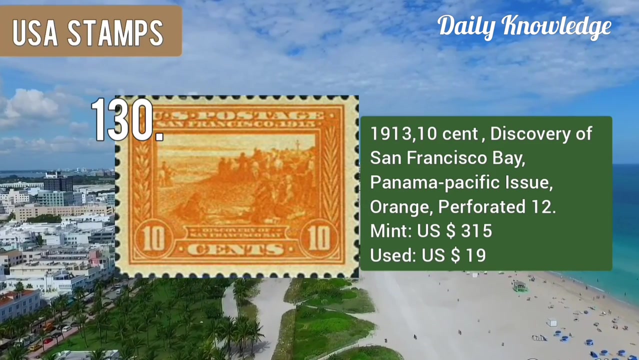 cent benjamin, franklin, blue, imbuffer ad issue. type two: missing lower balls 1909. two cent alaska, yukon, william h seward commemorative issue. now 1909. two cent hudson fulton commemorative issue and it is imperfect. in the last is 1913 tencent discovery of san francisco bay, panama, specific issue. 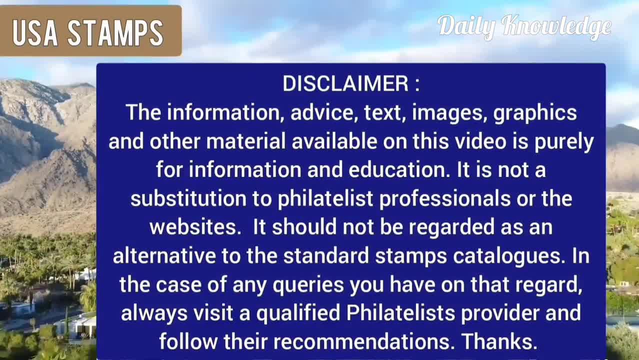 orange color and perforated 12. okay, friends, thanks for watching.